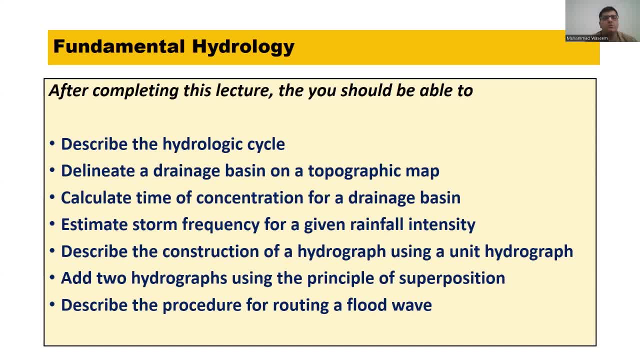 applications and how we can quantify that parameter. So this includes the basics, And then we will find the return period and storm frequency for a given rainfall intensity And we will study some similar stuff regarding the rainfall. And then we'll describe the construction of a hydrocarb, which is basically a pillar of hydrology, And we will study by using unit. 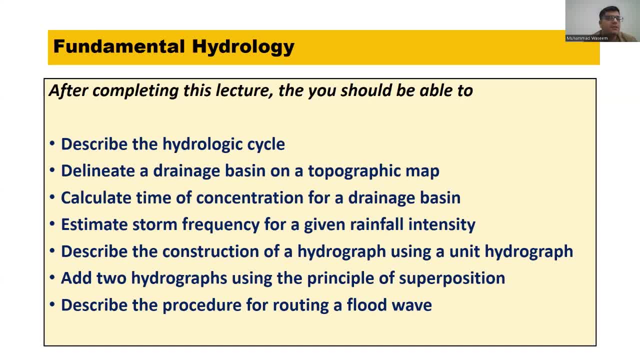 hydrographs And we will do some numericals, where we'll prepare some hydrographs, And then we will study the principle of superposition and the principle of proportionality which we use in preparing the unit hydrographs. And then, finally, in this chapter, we will study about 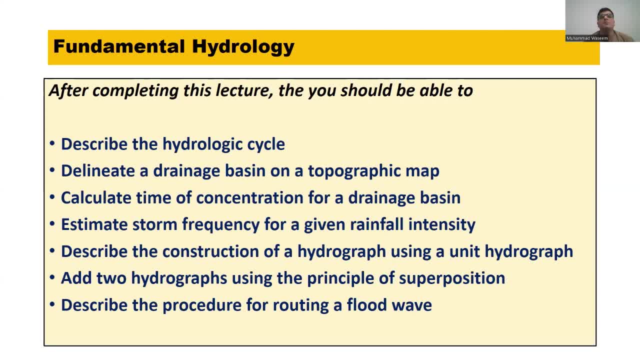 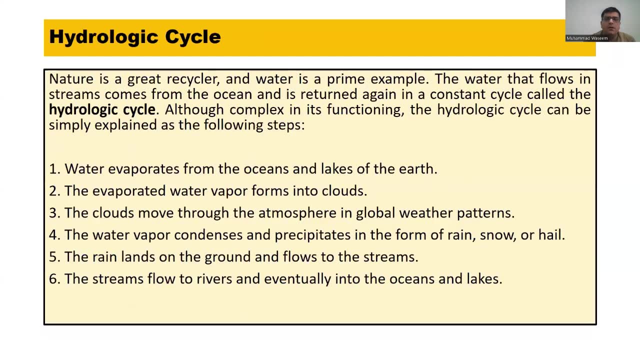 routing of flood wave. So this is basically the content of this lecture. After this lecture, you will be able to tell me the drainage basin based on topographic map, And we will do some numericals to understand these topics. So first thing first. so first thing is basically: 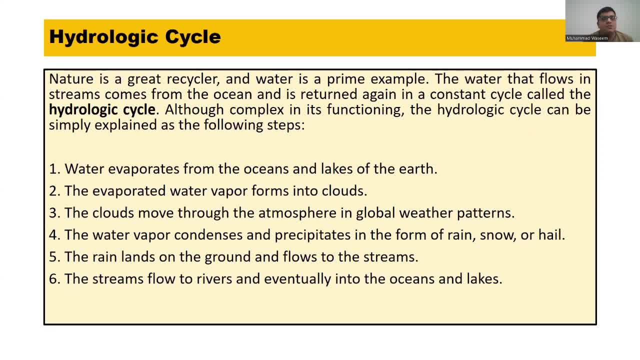 the hydrological cycle. So we know that nature is a great recycler, and the water is a fine example. The water that flows in streams comes from the oceans and is returned again in a constant cycle called the hydrological cycle. right In school we studied that okay, water evaporates from the 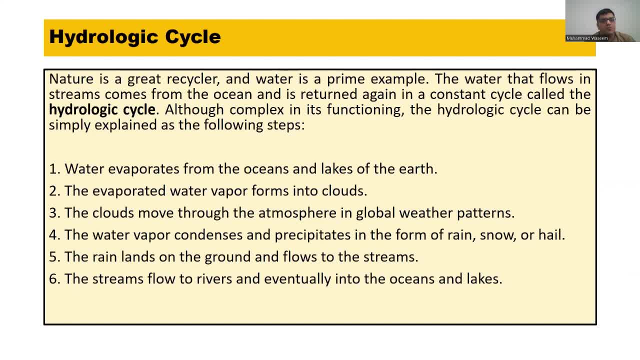 oceans and lakes of the earth. And then this evaporated water vapors forms into the cloud. And then, when these clouds, like, move through the atmosphere in different global weather patterns, the water vapor condenses and precipitates in the form of rain, snow or hail. Then the rain lands. 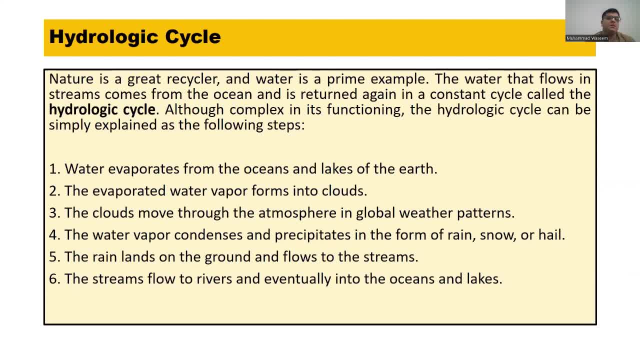 on the grounds and flows to the stream and then stream flows. All right, Thank you so much. Thank you so much. Thank you so much for your time. Thank you very much. 1600 questions to stop that from a standard here. 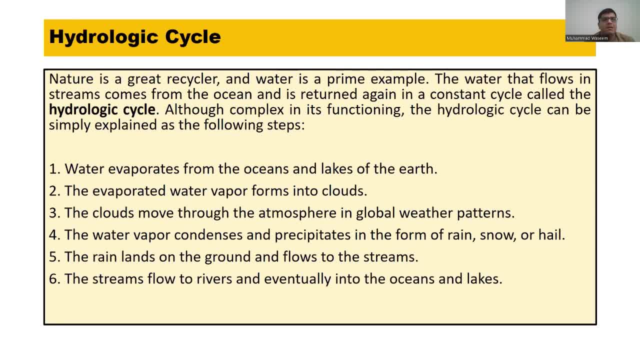 Let me just get back to pre- Reynolds Spencer. so we have narrow survey. what we are doing is we have rocky, briefly for retirementDa plus 20, 2007,. is this said in cities? So desert? because I like the term desert, because there's an image of that plan as fact. 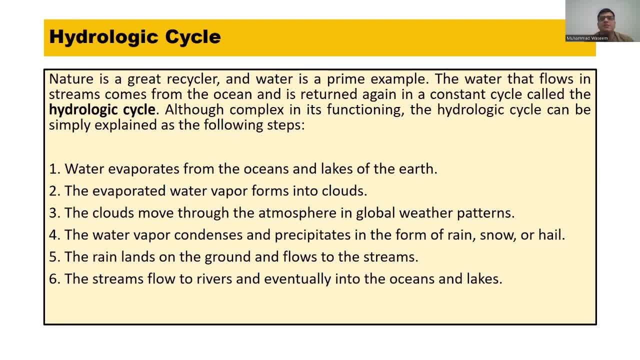 why is it said in cities? do they, for example, representation. This is called the weather Like. you cannot say that the weather of this, like 50 years of this area is like this. You can only predict the weather for like one week or 10 days, But in terms of climate, climate is basically the long-term representation. 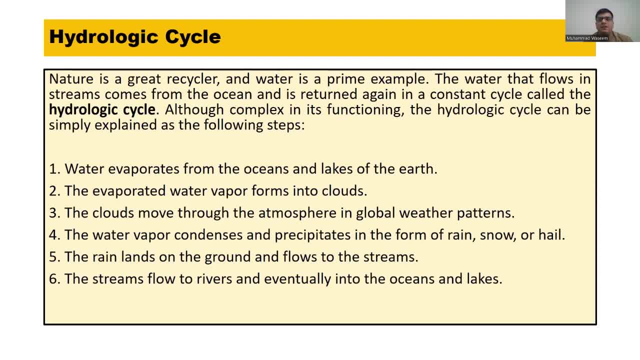 of a particular area. Let's say the climate of this area is humid. It means that it is based on like historical data, that is, maybe somewhere like 50 years or 100 years data, But for weather it's a short-term representation, like in terms of days or weeks, And the climate is the 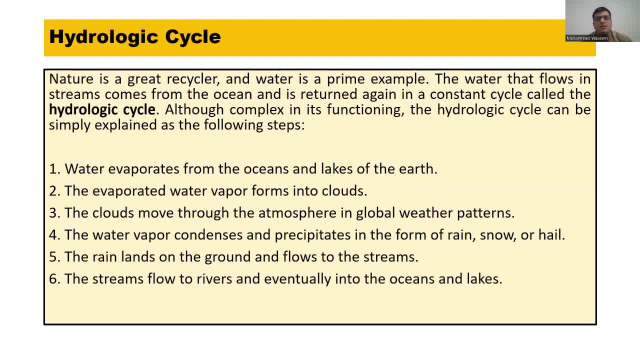 representation in a long-term representation, like in four decades. So in hydrological cycle this is like we know, that water evaporates and then it forms clouds And then, when the clouds condense, then it precipitates in the form of rain soon. 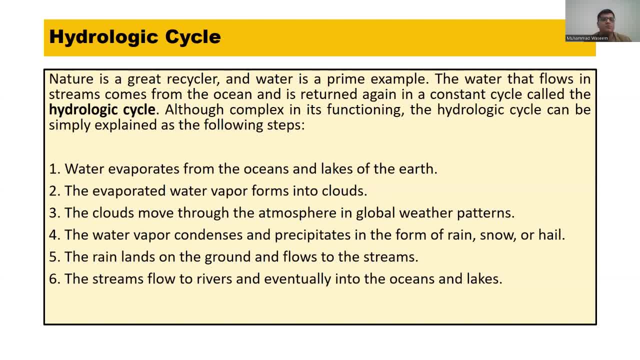 And then this rain lands on the government roads, to the streams And then, finally, these streams move into the lakes and oceans. So now here in this diagram- it will be easy to understand- You can see some things that are not listed in the diagram and what they are. 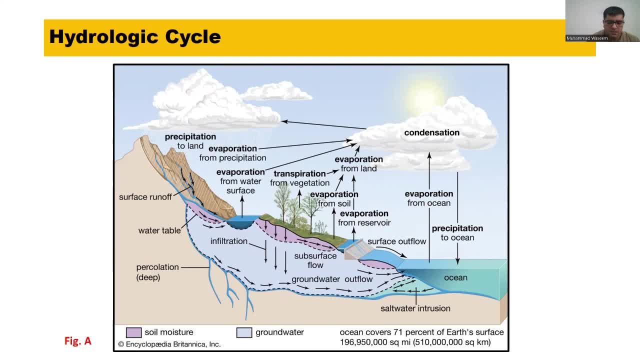 see, this is like here is, here is our chaos. okay, then there will be a precipitation. so this is like the precipitation: the precipitation happens, then some of the flow, then there is some water that will flow on the surface right- this is called the surface runoff- right and then there. 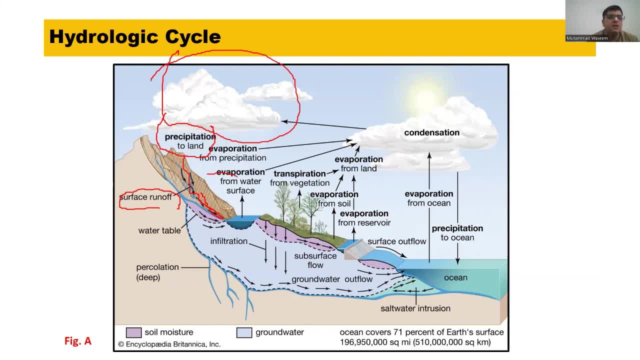 will be some infiltration and then this surface runoff will move to the open bodies like lakes or rivers, and then there will be some evaporation from water surface right and then some of the water will be infiltrated from these open surfaces and if it moves in, the unsaturated 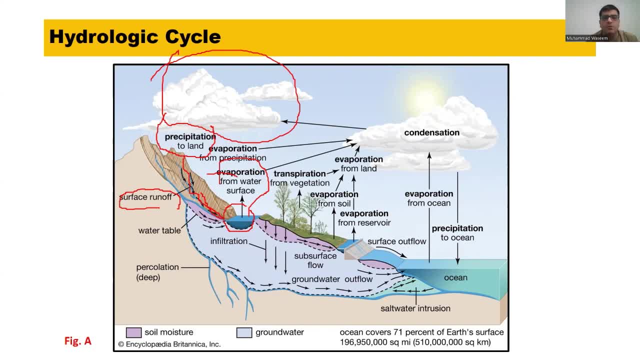 zone subsurface to the nearest, like river or ocean, then it is called the subsurface flow. let's say, if it goes deep and and becomes the part of the ground water, then it is called the percolation, like if the infiltration is like the water infiltrates at the surface and when that 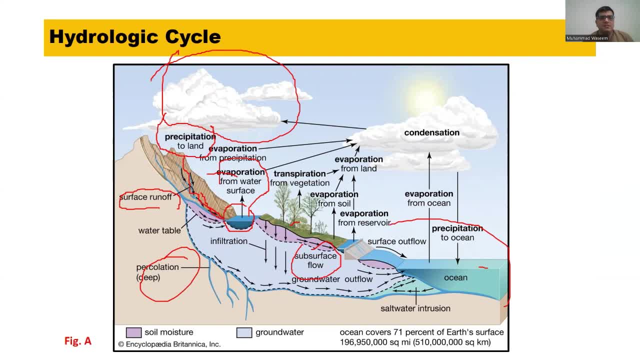 infiltration literally moves, then it is called in the unsaturated zone, which is called the subsurface flow. but if that water, infiltrated water, becomes the part of of ground water, like there is a deep vertical infiltration, then this process called the uh, like percolation, that. 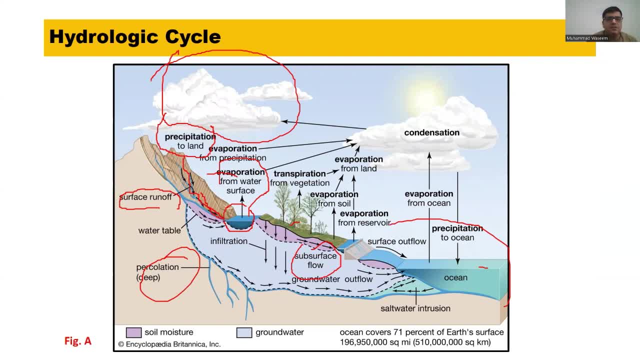 that moves deeply. it's basically the deep percolation and then everything like the ground water flow moves towards the lowest points. but the speed of the ground water, the velocity of groundwater movement, is very low, like one to two meters per day. so here you can also see that uh. 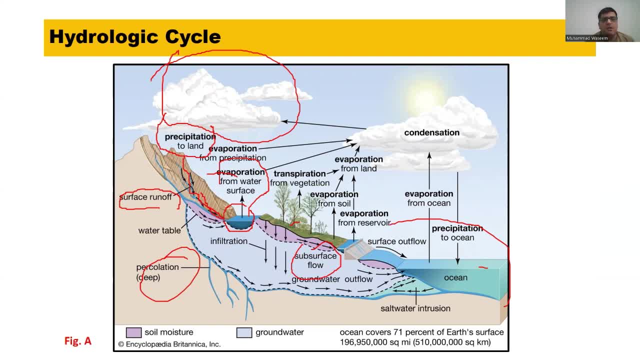 evaporation and then transport, transpiration, uh terms. so here is the transpiration. so evaporation is normally the vaporization of water, uh from liquid to gas from the open surfaces, but the transpiration is basically the evaporation that happens from the leaves of the vegetation or or any trees. so this, this is called the transpiration. 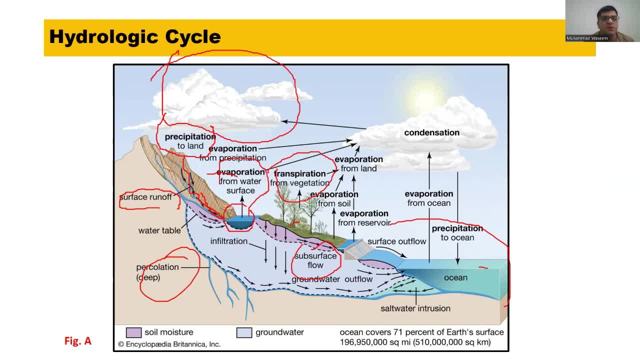 so when we talk about evapotranspiration, so this is basically the combination of evaporation and transpiration, right? so here is also a one phenomena explained here as sea water in korean. so this is, uh, this is the reason that we we need to send fresh water into the ocean. 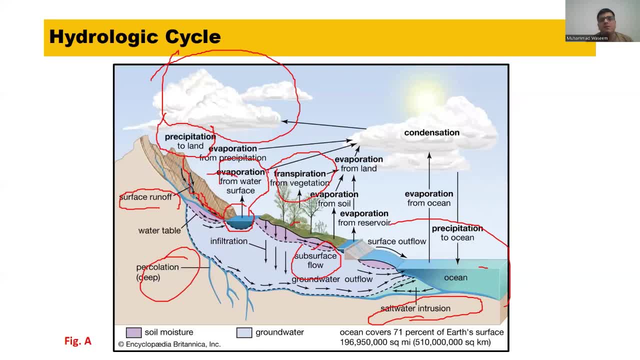 uh, because we don't want that ocean travels towards our- uh, fresh water resources are towards our groundwater. that's the reason that in in in coastal cities like in Karachi in Pakistan, there is no drinking water. the gum water is like salty, because there is a seawater. 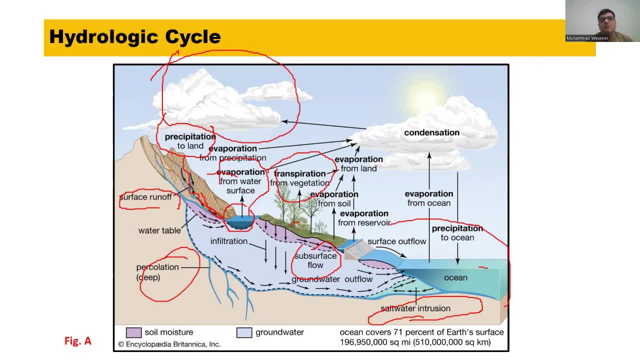 and although we are discharging a much larger amount of water into the sea, but due to lack of uh management. this there is a sea water, including phenomena, that that sea is moving towards the cities and towards groundwater and it includes our groundwater and that's why there is uh there. 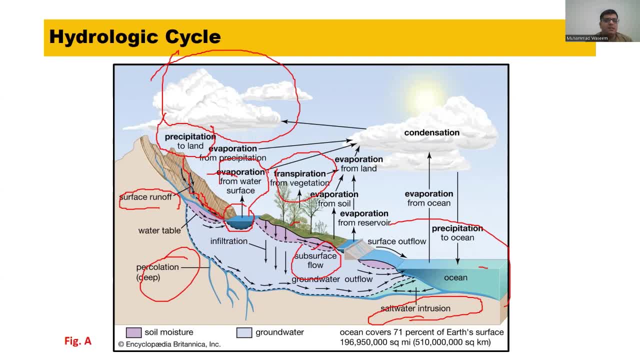 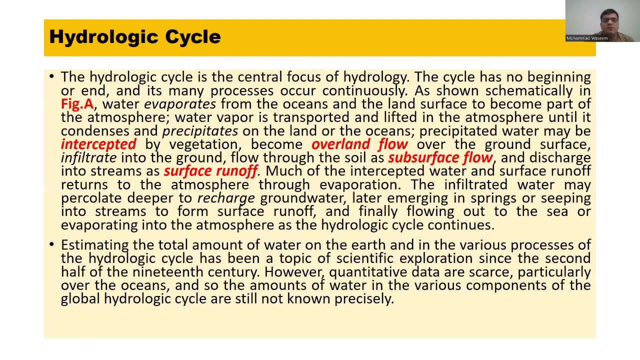 is an issue of of drinking water in in mainly in coastal cities, if there is a lack of management. so and the basics of hydrological cycle, so in uh, the Hydrological cycle uh, in terms of explanation, is the central, central focus of Hydrology. you need to know the um, Overland flows, subsurface flow and 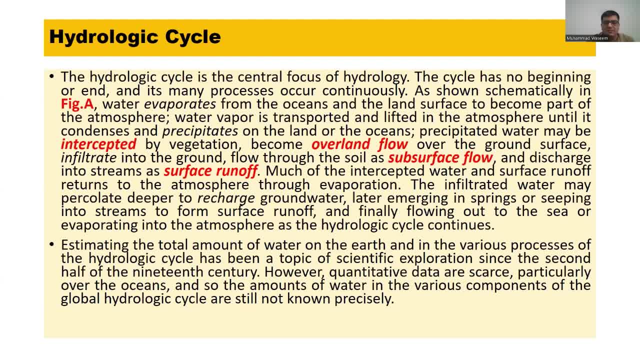 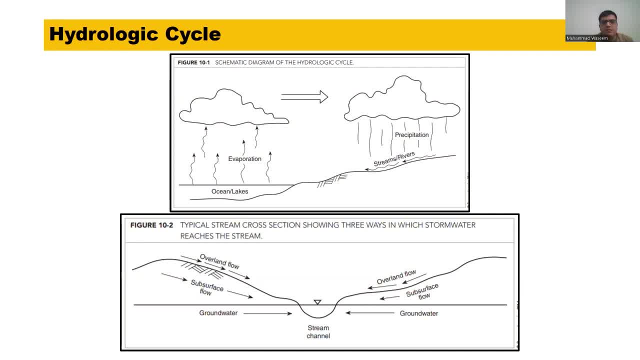 surface runoff. so, uh, to understand these things, let me go to the next slides. here you can see when there is a precipitation. when there is the precipitation, there is some water that will move the surface. that is called the overland flow or surface runoff. in different books, the different 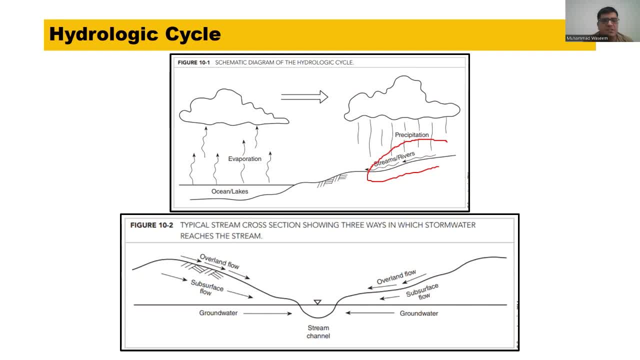 terminologies will be used. sometimes it's called well and flow, sometime it is called surface runoff. so so you need to understand this thing. that's why i have added the slides from two different books. so the water that will infiltrates, that infiltrates and and move towards the lowest point. 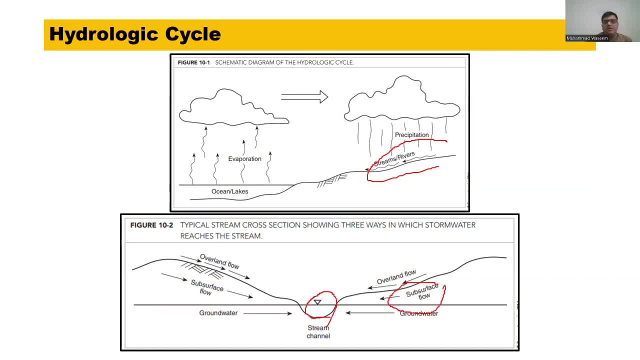 so the lowest points are our rivers or any natural streams and move towards it in the unsaturated zone. the later moment, then this flow is called the subsurface flow, and when it becomes the part of groundwater due to the phenomenon of population, then it's also towards our streams. so sometimes 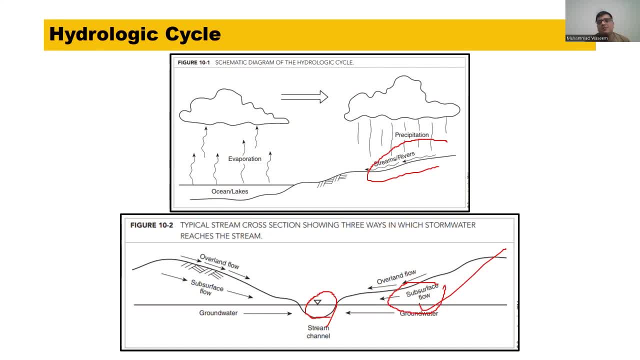 our groundwater contribute to our streams, and in lowlands, in highlands, the streams contribute to our groundwater and in lowlands, groundwater sometimes contribute to our stream, so so there is always an interaction between between the filtration from the streams and the groundwater contribution to that stream. so here we up till now. i i believe that you know basically what is. 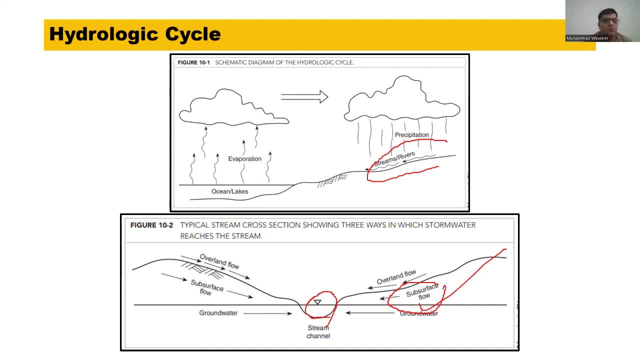 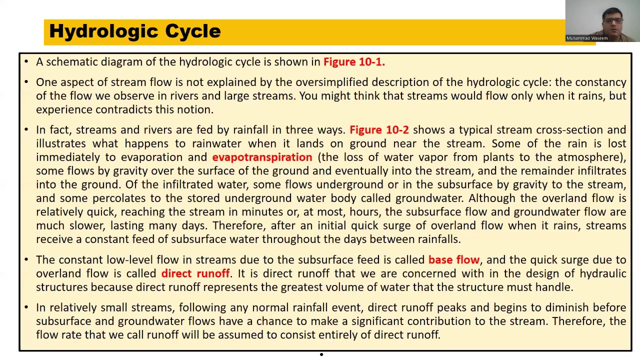 the overland flow, what is subsurface flow? what is groundwater? what is transpiration? what is evaporation? what is the vapor transpiration and the, the, the government, what is the speed of groundwater? so this is the basic, basic thing which i want, that at this point you need to know. so then the hydrological cycle, these basic terms of 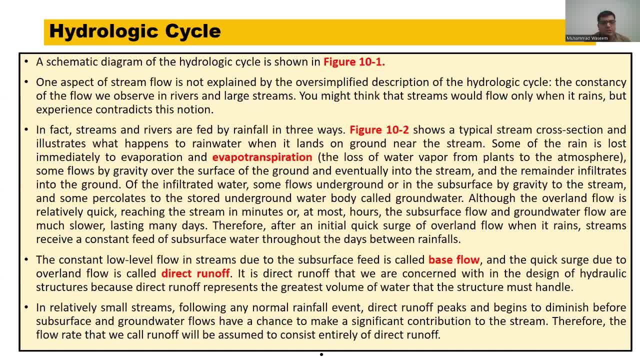 transpiration, then the ones in the red: the base when the red runoff. i have explained you in the previous slides by showing you that the the representation of an image of the hydrological cycle. so next thing, so next thing. basically, i would like to tell you that is the. 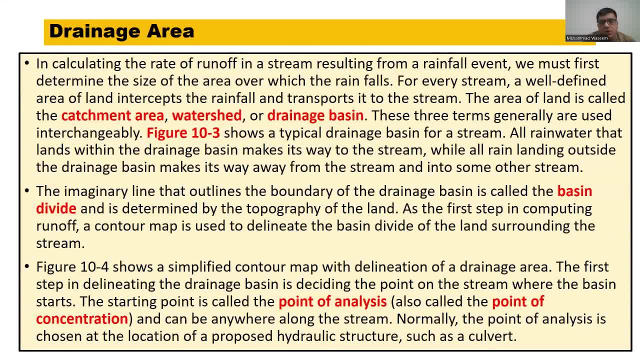 drainage area. let's say, when we talk about hydrology and, and and you want to do some hydrological analysis, you always talk about the, the, the catchment area or drainage area. so the drainage area, or catchment, or basin or a watershed, this is basically uh, uh, one name, uh the different. 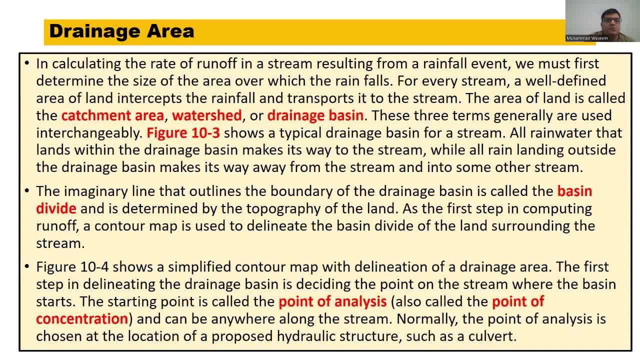 names for uh one one, one thing. so uh here, uh, if, if you want to uh remember the definition of a catchment area: watershed or drainage basin, the area that contributes water, the area that contributes water to a river is called its catchment. right, so how we uh, how we um delineate the catchment? we delineate the catchment based on: 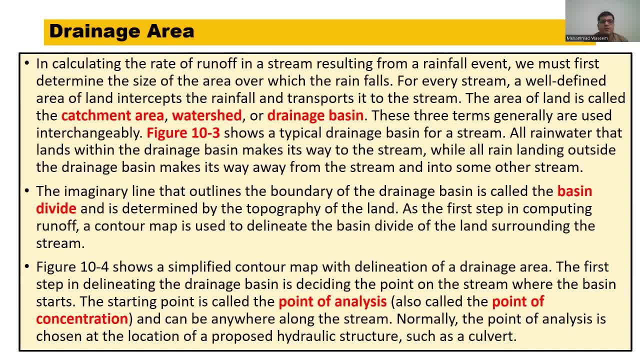 the topographic contours, we imagine that the rain of the rainfall drops, then in which direction it travels. so normally, uh, the rainfall will travel perpendicular to that at each point, perpendicular to the control lines. so, and when we uh study about the hydrographs- we will study in the next slides- 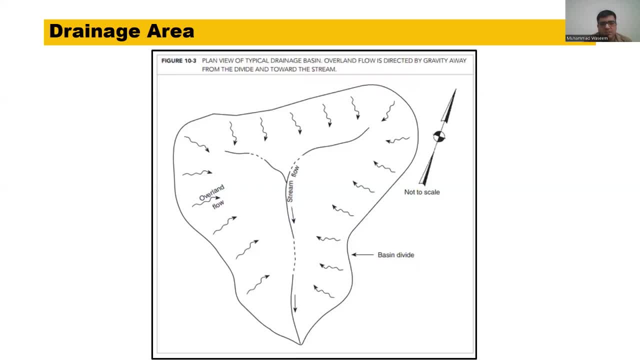 we always calculate the hydrograph at the point of analysis. so this is basically the streams, the stream, and then this is the area which contributes to that river if there is a rainfall as a surface flow. so this is called the catchment area of that particular river and there is the boundary which divides this particular catchment from the other catchment. 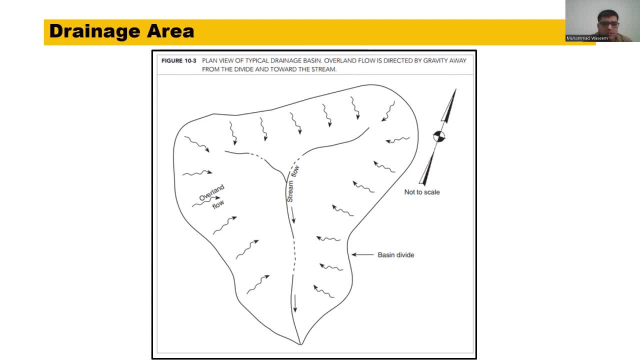 is called the basin divide, and this point, basically this point, is the point of analysis where, uh, we study all the stuff like the flow gauge, or how we measure the one major differences, like hydrograph. so now, next slide is basically about the time of concentration. let's say, in this particular train, uh, catchment, there is a rainfall. 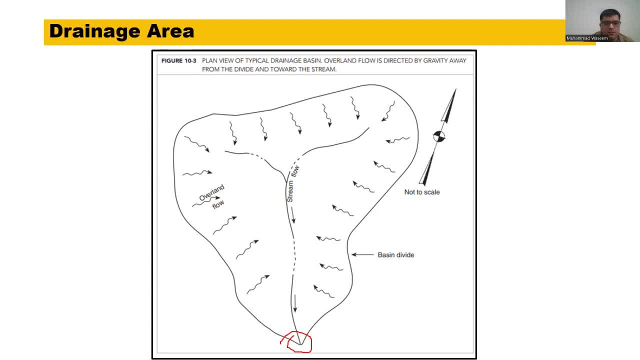 there will be rainfall, in the rainfall, over the entire area, right and then sorry, uh, and then you. so time of concentration is basically that from from the remotest point, the time it takes for the rainfall or water to travel from the remote point to the point of analysis. this is basically the time of concentration. so now there are 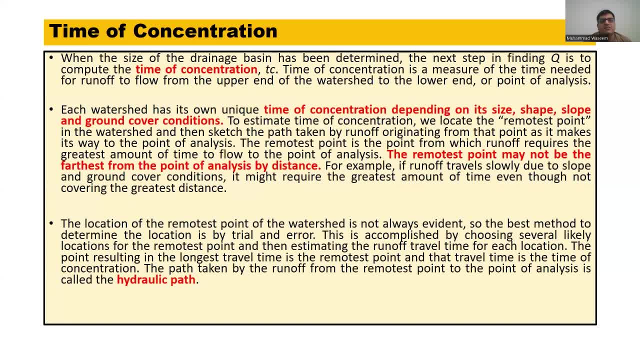 different things. let's say first, when the size of drainage basin has been determined from the delineation of the catchment, the next step in finding the q is basically the discharge is the time of concentration. so the time of concentration is the measure of time needed for the runoff to 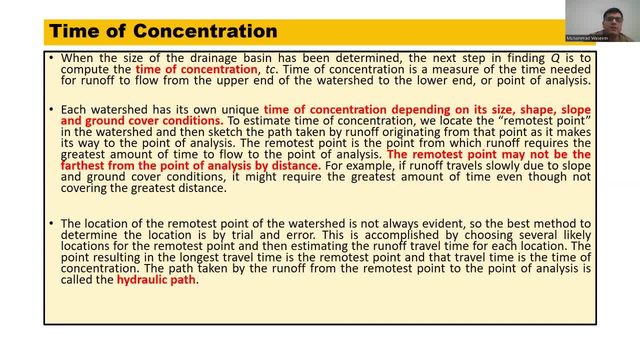 flow from the upper end of the watershed to the lower end or point of analysis. right upper end means the remotest one. each watershed has its own unique time of concentration because it depends on the size, shape, slope and groundwater conditions. to estimate time of concentration will indicate. 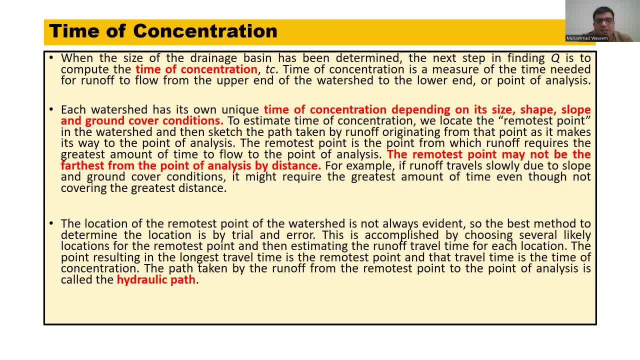 the remotest point in the watershed. but you need to remember that that remotest point may not be the furthest point from the point of analysis by distance, for example, let's say if we are on the ground of travel slowly due to slope and ground cover conditions, it might require the greatest. 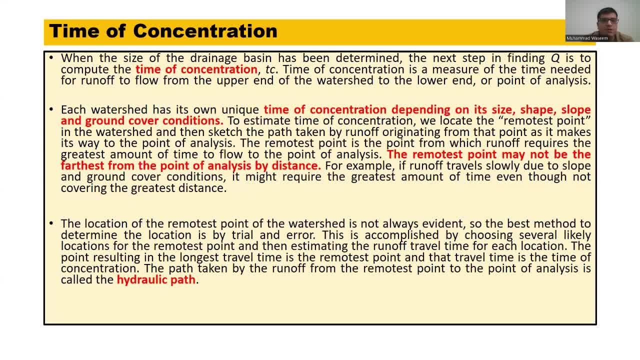 amount of time, even though not covering the great resistance and the and the and the run of the paths, which is this is taken by. the runoff is called the hydraulic path, right, so you need to remember that the remotest point on ground distance may not be the remotest point that you will analyze for the. 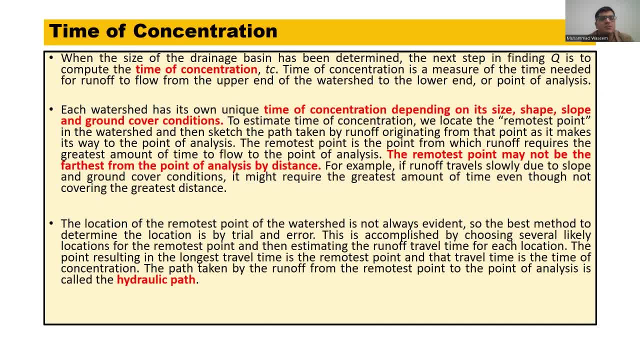 penetration. you need to know that, that it depends on the size, it depends on the slope, ground cover conditions. let's say, if there is a sandy soil, then there will be less surface runoff and more infiltration, right, if there is a, if there is like a paved surface, there will be no. 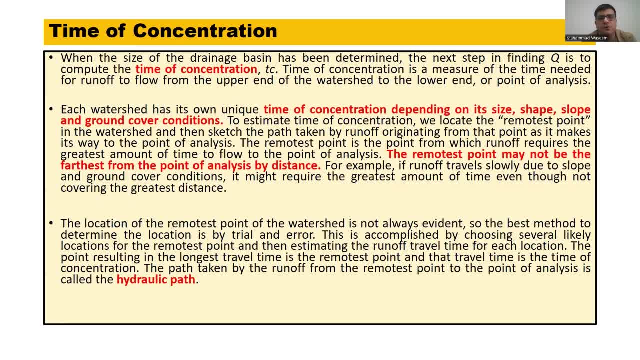 infiltration- not really no very minute infiltration and maximum surface runoff. so uh, so uh. if the point which is like very near but it's not paved, it will take more time for the runoff to to move towards the point of analysis. but if the remotest point, the path is like paved to the point. 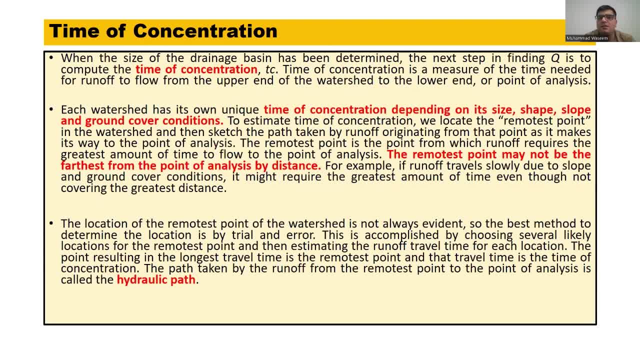 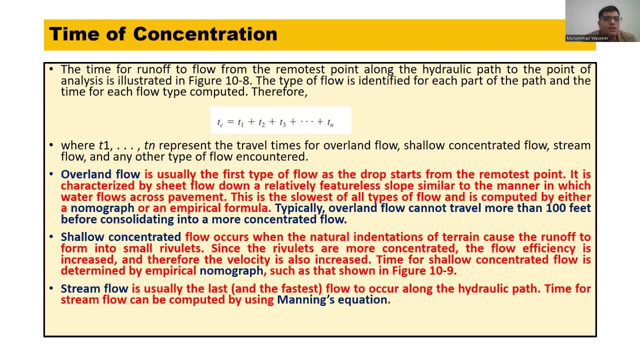 of analysis, then it will not be the uh, it will not serve as the point to calculate the time of concentration. so you need to know from which point it takes maximum time to reach the surface runoff to the point of analysis. so, uh, the time runoff from the remotest point along the hydraulic part to the point of analysis. 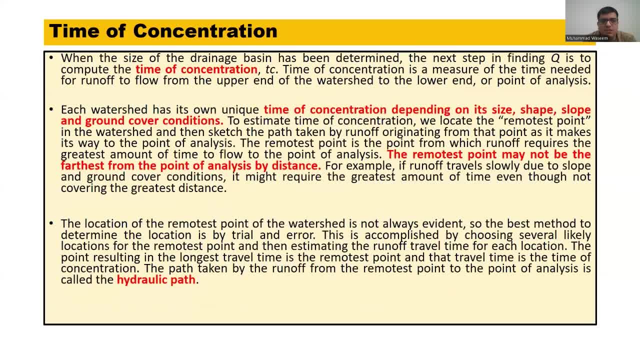 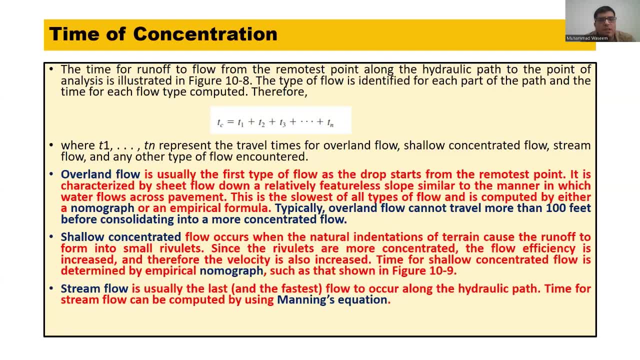 uh is illustrated, uh, in the figure 10-8. i will show you the figure 10-8. uh, this type of flow is identified for each path. we will try to cover one example too. and then you add all these uh times for overland flow, for shallow, concentrated co-answering flow. so let's say: 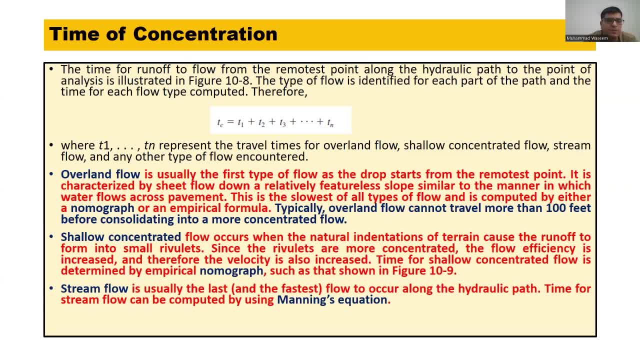 a big valley flow and uh, be okay. moreguys orATHER say that now overland flow will not be the overland flow because, um, the rain won't, or always. the rate of non- pross Tenant flow will be changeable if the flow percentage is. 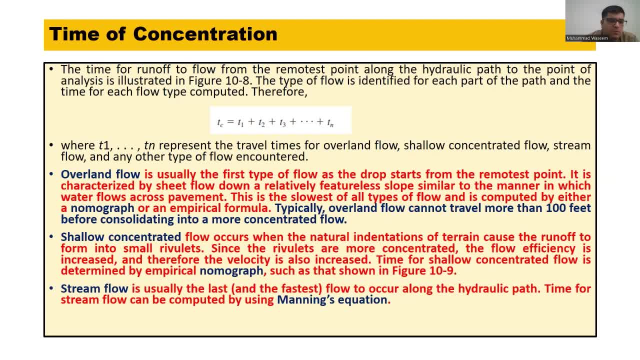 very high and again, only this ge Avecal is available in high credited flow, more concentrated and then shallow concentrated flow that the flows becomes into small rivulets and then in stream flow, these all rivulets merge and become a stream or a river right. so you need to remember that. 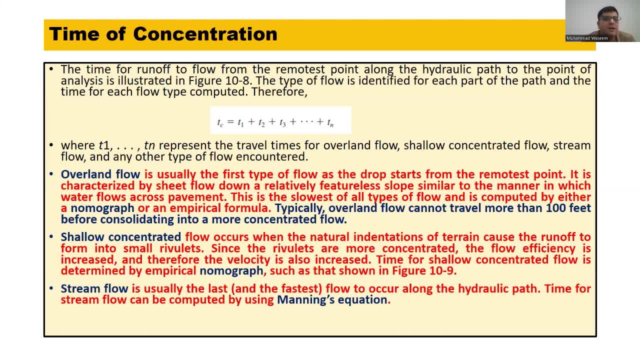 overland flow: uh, the time of concentration is measured by a nomograph. shallow concentrated flow. you can also determine by nomographs, or we have some, uh, some graphs, and for stream flow we we can use the main equation. so how to study the nomograph, i will explain in the next slide. 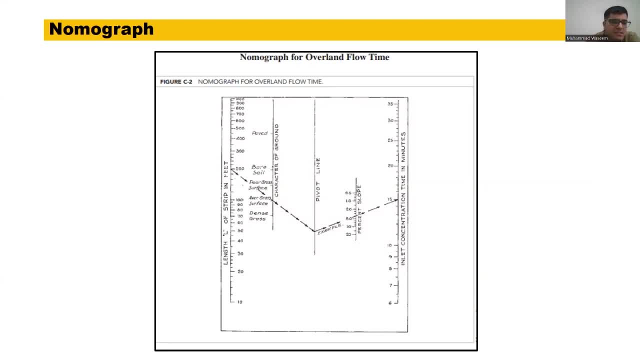 so this is basically the nomograph. let's say: uh, you have a strip of uh 100 meter uh, and the average and the land use is average gas and the slope is like uh two percent, so what will be the time of concentration? so let's say so what you need to do. 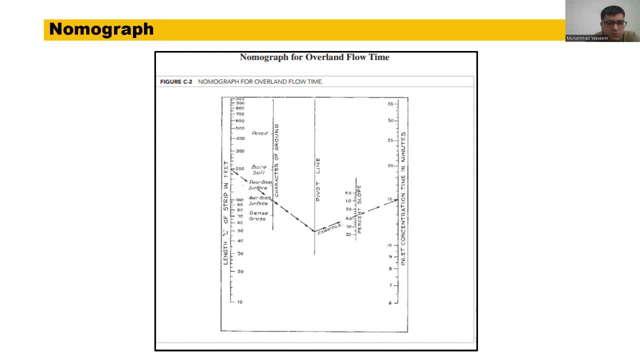 is form 100 to. you will come straight to the average gas, which is the land cover, and you will come straight to the pivot line. and then you will go from this point to the slope- our slope was two percent- and you will come straight. sorry, i couldn't draw the straight line, but you, you need to go to the 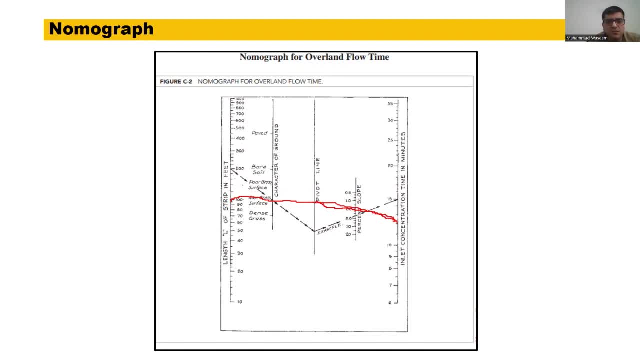 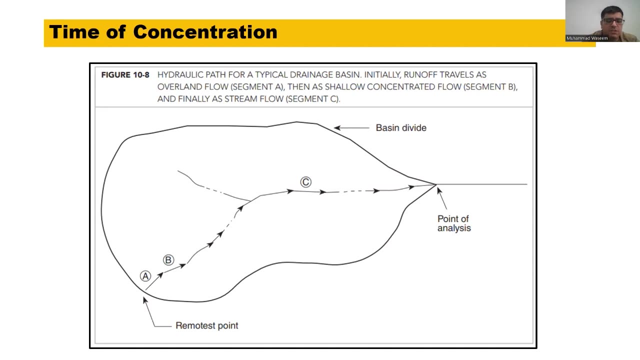 straight line, uh, straight. so it will be somewhere 10, 11 and 12. 12 minutes will be that time of concentration. so this is how you study the nomograph. so this is then the shape figure. here you can see the remotest point. so initially, 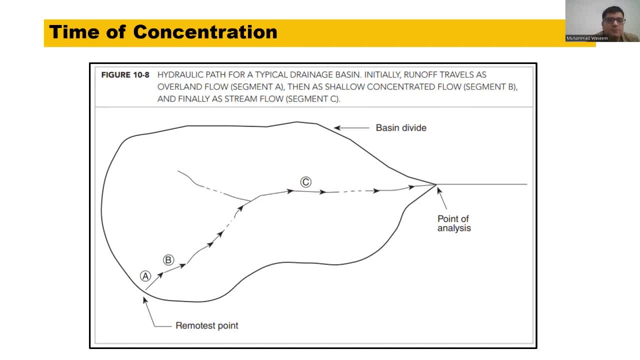 flow type a. flow type a is basically you. you know the initial flow will be overland flow, so there is overland flow, and in b it is basically the uh, shallow concentrated flow, and when then shallow concentrated flow will go, will change into the stream flow for 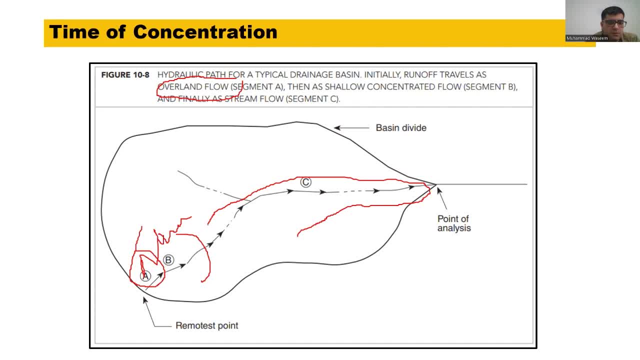 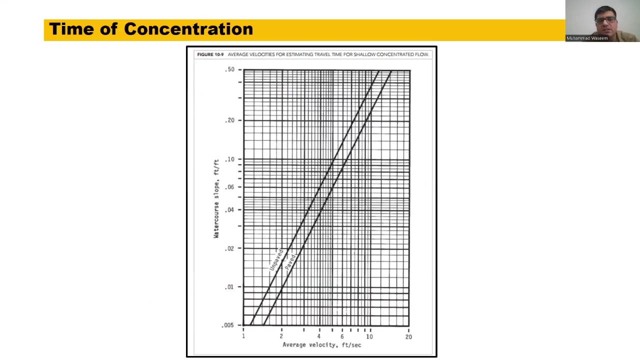 overland flow nomograph for shallow concentrated flow. we can use the nomograph for some other graphs and for stream flow we'll use the manning equation. so this is also one graph. average velocity is for estimating the double time for shallow concentrated flow. these kind of graphs we can use where we can. for average velocity we can find the 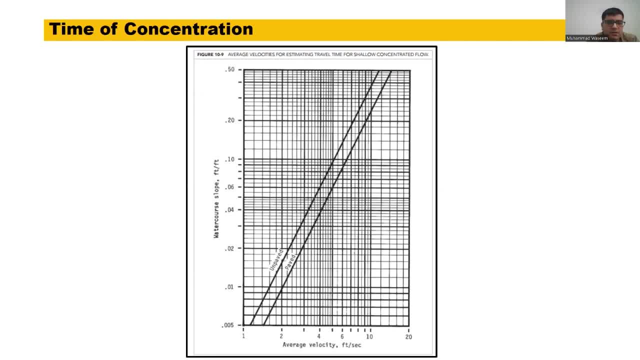 uh, uh. for you can see if we have watershed slope and if you know the land use, then we can find the average velocity and then from this velocity we can find the time of concentration. we will solve one numerical, then all these things will be get more clear. so here: determine the time of. 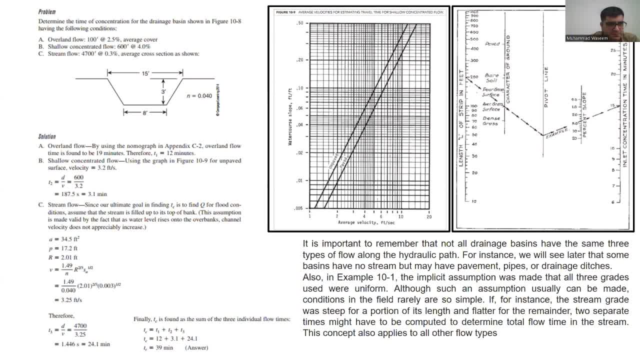 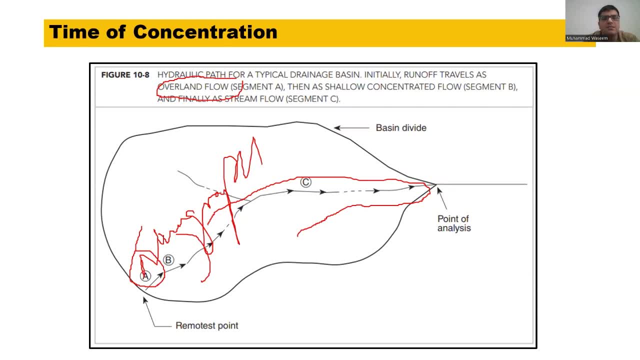 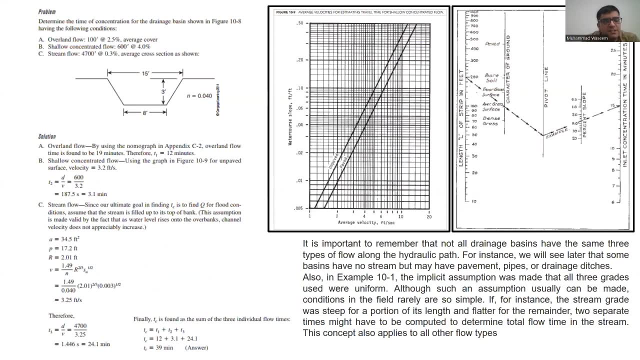 concentration for a drainage basin shown in figure 10-8. this was basically 10-8. this way, initially there is a uh overland flow, then there is a shallow concentrated flow and then finally it is a stream flow. so here overland flow is 100 feet. uh 2.5 average cross cover. 2.5 percent is the 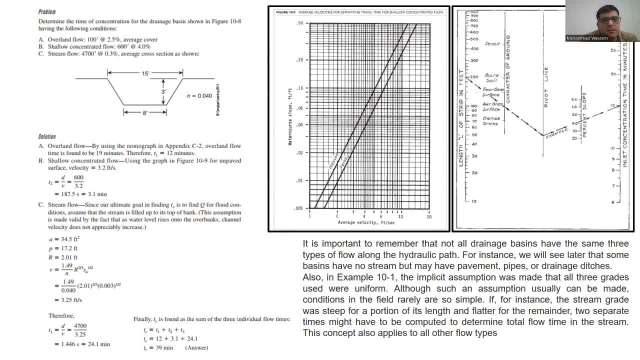 slope, then shallow concentrated flow: 600 feet and four percent uh slope and then stream flow is 4700 with 0.3 percent average cross section, as shown in figure. so now, first thing, overland flow, so overland flow, uh. the given data is that 100 feet and 2.5 percent slope and average cross cover. so 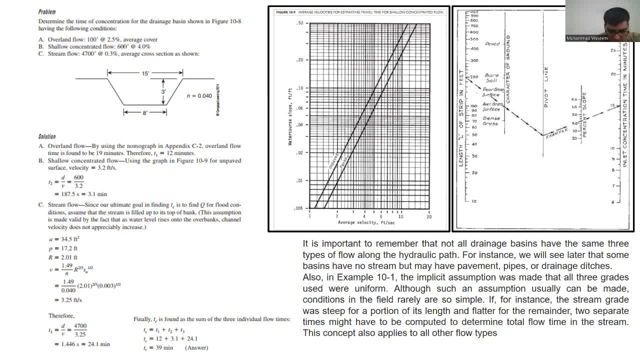 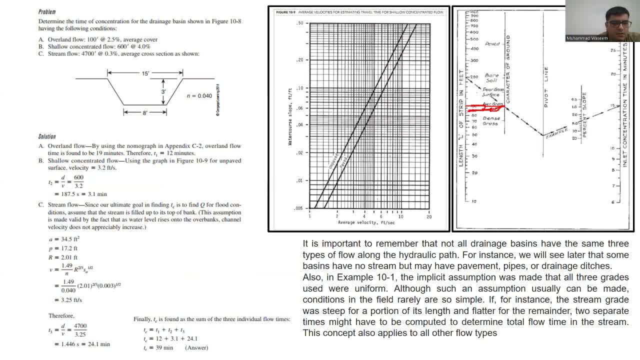 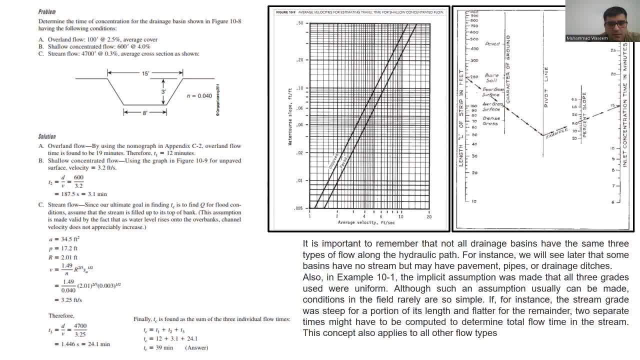 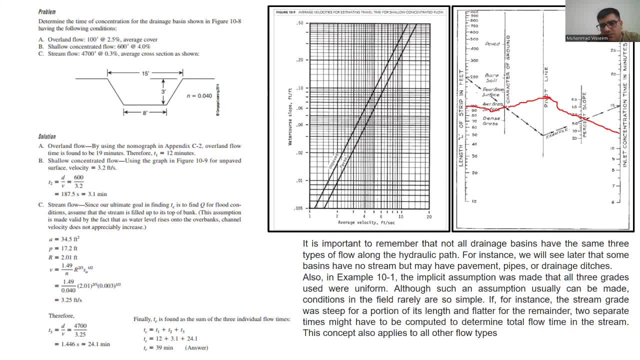 so this thing, and you will take straight into the pivot point and then give it to. for the 200 feet average grass, you came here like in a straight line, and then for the slope, you intercept the slope and extrapolate it towards the time of concentration. so in this case we get the 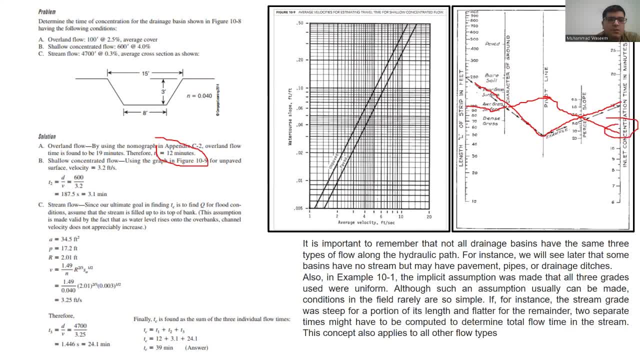 12 minutes. this is somewhere here. 12 minutes for our land flow. now for shallow concentrated flow, uh, for unpaved surfaces, uh, the the velocity is 3.2 feet per second, which we got from this, this graph. how we got this, we i will explain you. so the given data is: it's a 600 feet. 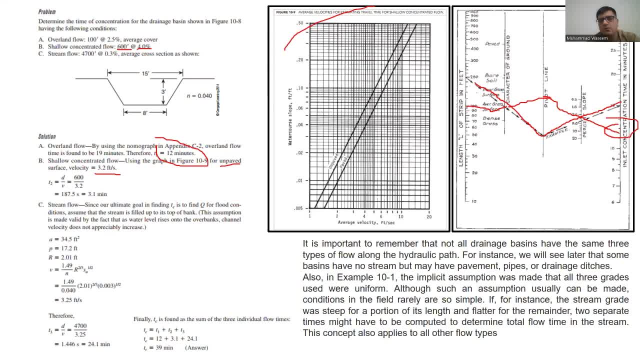 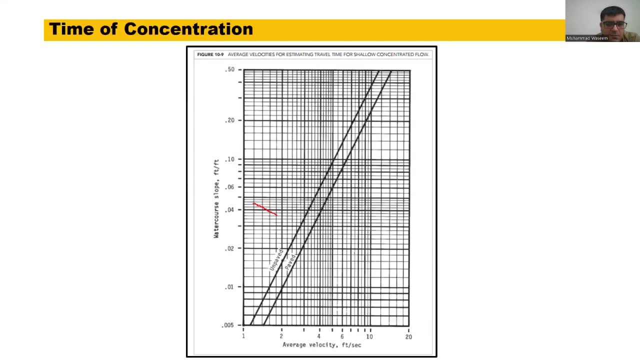 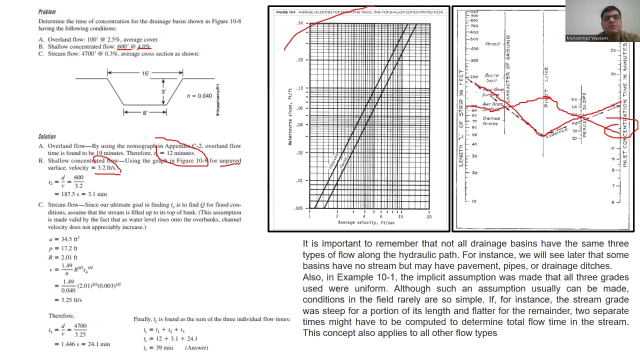 path length and four percent slow. so here it is small, i will go there. so it was 600 feet and four percent slow, so slope is four percent. it is is unpaved. so here you will find something, the velocity per second. so it was 3.2 feet per second the velocity, and you know that time is distance over velocity. so 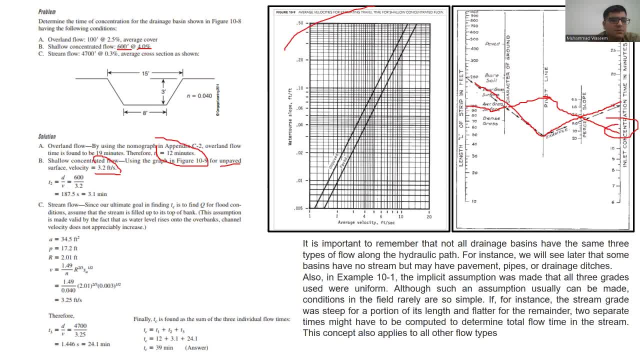 basically 600, which was the distance, and the velocity is 3.2 feet per second and you will get the time of concentration for shallow concentrated flow as 3.1 minute. then there is a stream flow and then you have a NEWR, Werner Green, Uh, Lerner. 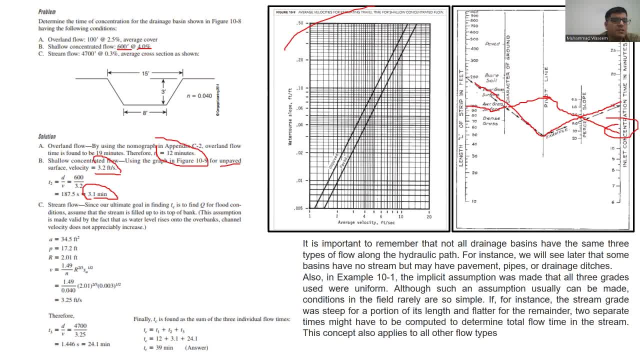 unku water level, S질 on that stream flow, one you can get now because we see the flow from this channel. we can find the area of this, uh. we can find the area of this, uh. we can find the area of this departments channel cross section. we know the. 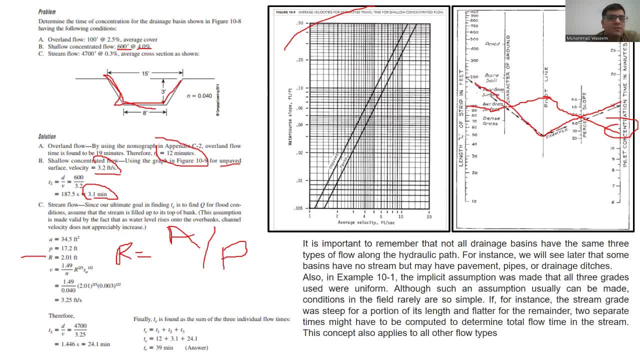 formula, as i have explained you in the previous slides, that to find the velocity we will, we will use the manning's equation, which is: v is equal to 1.49 over n, r raised to power 2 by 3 and s raised to power 1 by 2, this s naught is basically the channel slope. so here you can see that the 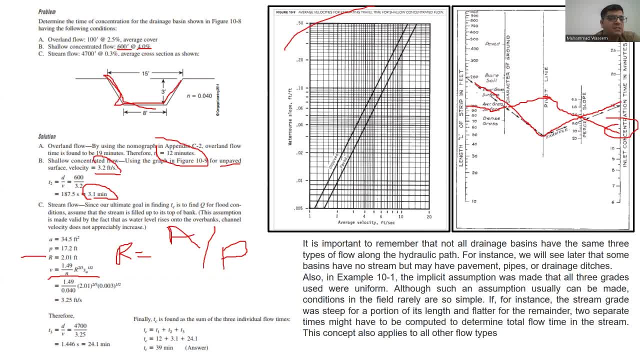 velocity dependent on n, which is basically the manning roughness coefficient, and r is the hydraulic radius, which is basically the cross-sectional area and the vector parameter and the bed slope. so the velocity is dependent on roughness, cross-sectional area, vector parameter and the bed slope of the channel. so from here we have find the time of concentration, the velocity and then 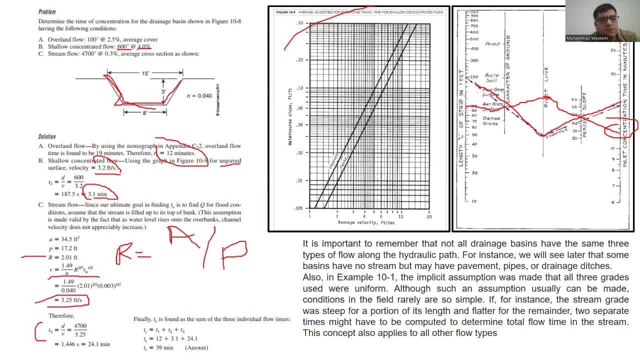 the time of concentration is basically the d over t, so the time of concentration for stream flow is 24.1 minute and then, finally, we will add all these times, then we will find the time of concentration at 39 minutes. but it is important to remember. 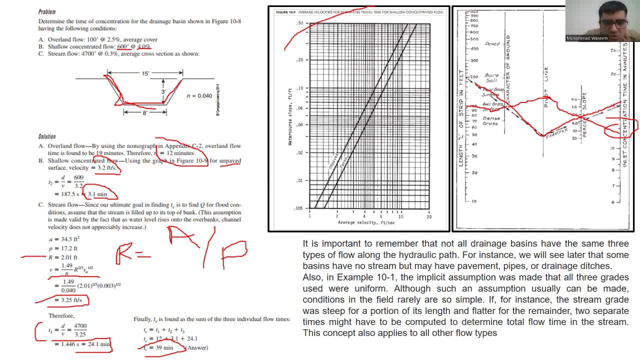 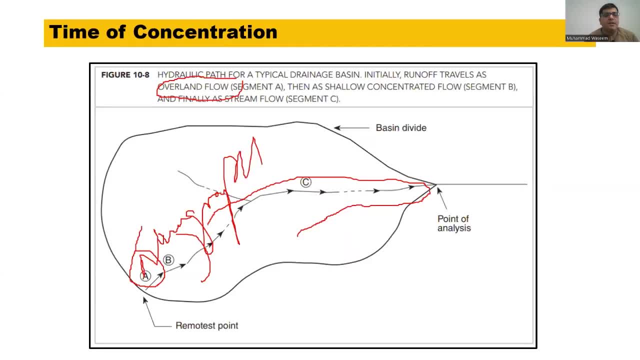 that not all the drainage basins have the same three types of flow along the flow path. here 10.8 you, we have said that in the whole, in the whole basin, the initially there is a whirlwind flow, then the shallow concentrated flow and then the uh stream flow, but in reality uh. 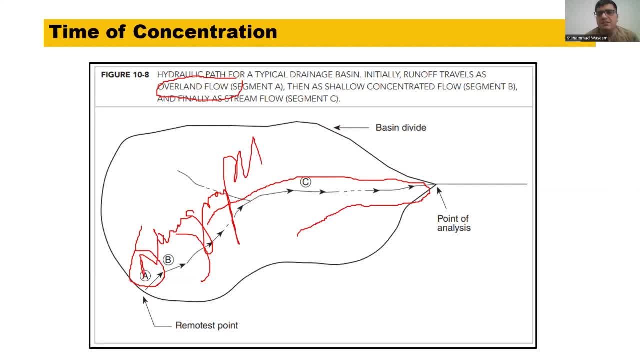 the, the conditions are not same for the whole drainage basin, then we have to divide the basin into sub-basins. we will study that later on in this lecture, that how we can divide the, the catchment area, into small sub-basins so that the conditions remains constant throughout the smaller portion. 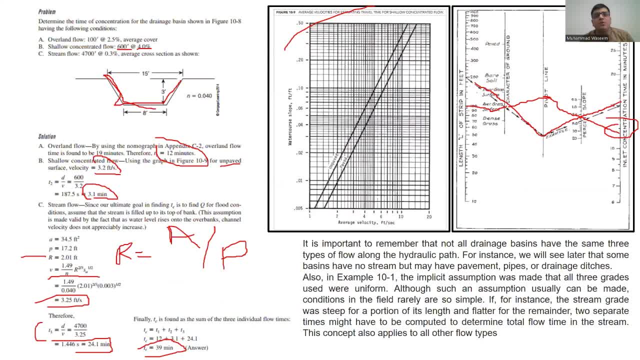 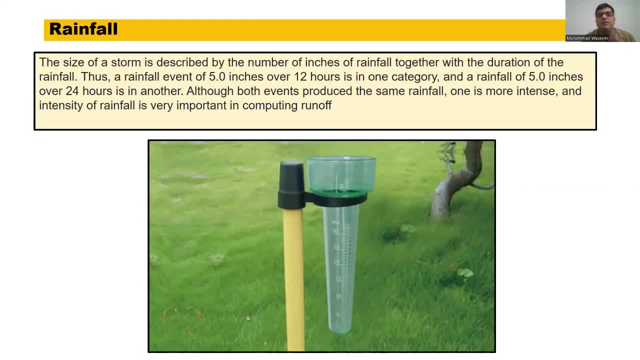 called sub-basin. so this we we know. and then now we move towards the rainfall. so, uh, we have explained the how it um rains when the clouds condense and then it precipitates in the form of snow and hail. so here is a typical range, and but here i would like to explain that what is basically? 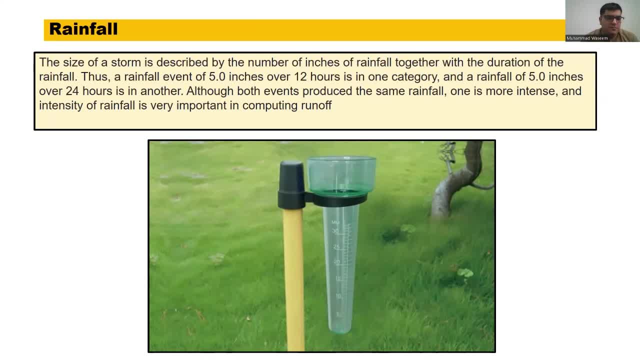 the intense rain or in comparison to a non-intense ring, let's say, a rainfall event of five inches over 12 hours in one category and a rainfall of five inches over 24 hours in another category. both these events produces the same rainfall. one is more intense, uh, and intensity of rainfall is. 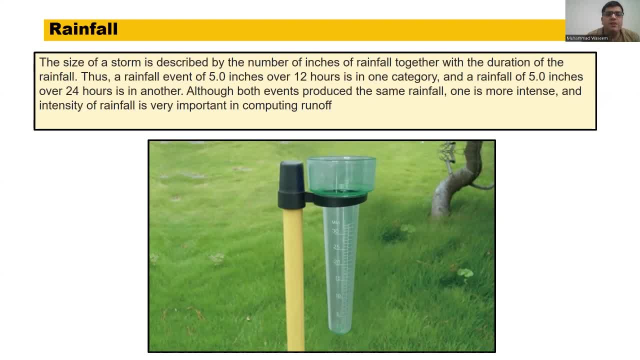 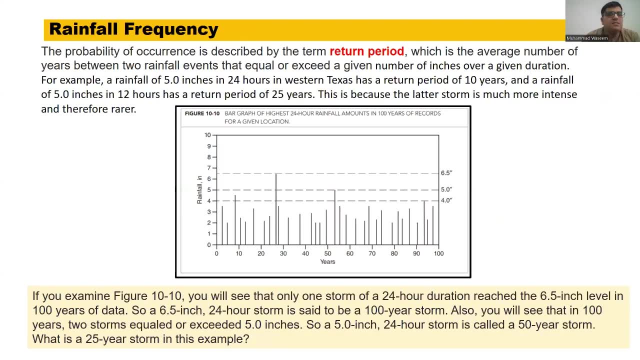 very important in computing the runoff. so when the rainfall of five inches happens in 12 hours- that is more intense storm- then we need to know the frequency or return period of rainfall. the probability of occurrence is described by the term return period, which is the average number of. 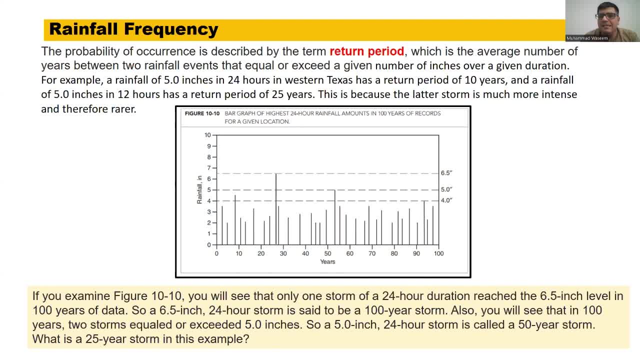 years between two rainfall events that equal or exceeds the number of inches over a given duration. for example, a rainfall of 5 inches in 24 hours in western texas has a return period of 10 years, and and a rainfall of 5 inches in 12 hours has a return period of 25 years right. 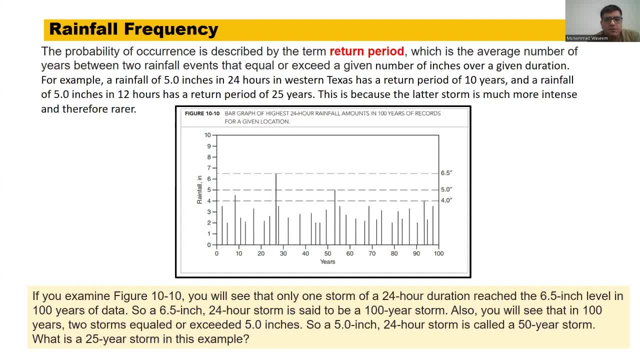 so here you can see that 5 inches in 24 hours. it has a return period: 10 years and a 5 inches in 12 hours in a smaller period, 5 inch rainfall. it has a return period of 20- 5 years because it it takes once in a 25 years that 5 inches rainfall happens in 12 hours. now, if 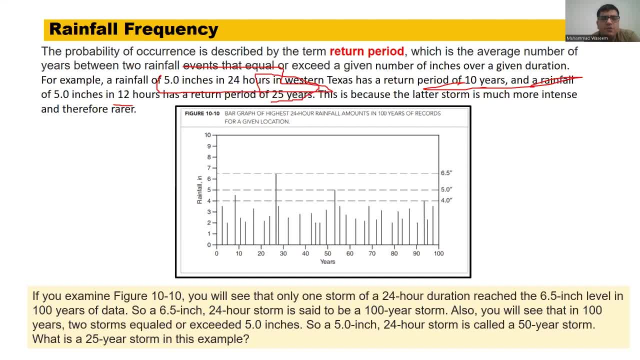 you study this graph here. if i say you what is the return period of the of the rainfall of 6.5 inches? here is the rainfall of 6.5 inches, this one. so you can see that in 100 years, this is basically years. it happens only once, it only happens once. so the return period this is a 100 year, storm 6.5. so let 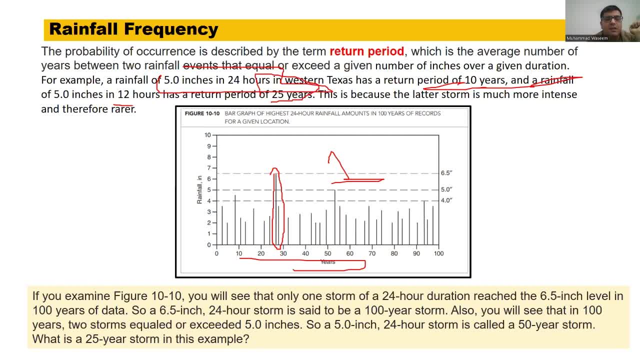 us say, uh, if, if. if. i say uh, five inch, if a storm that equals or exceeds five inches, what is the return period? so you can see this, and this is the one time and this is the second time: equal or exceeds. so we can say: this is basically the 50 years strong. so if, if a particular rainfall equal 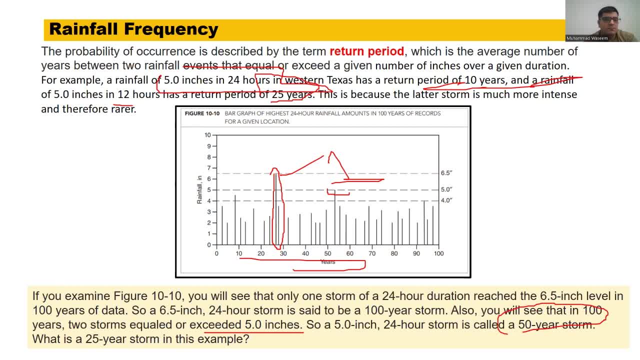 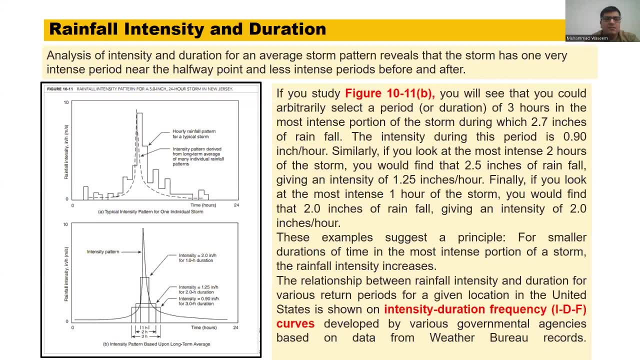 or exceeds three times, then it is called the uh, like you can say that it is equal or exceeds three, 33, 33 year storms. so now the next is the rainfall intensity and duration. in this graph you can see, as, let's say, this is basically a typical uh hourly rainfall pattern and this is 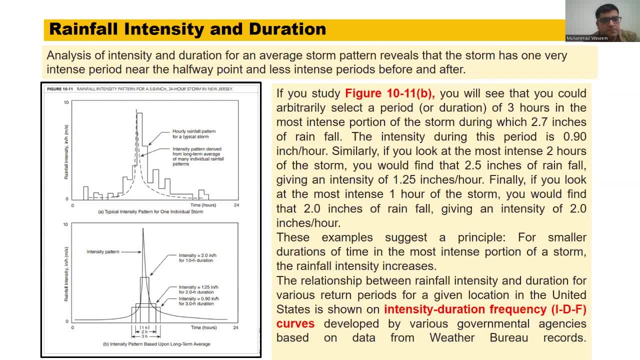 basically the intensity pattern derived from the long historical data. if you move towards the center of our involvement, right, it will be always intense, and if and then it's intensity will be lower, right? so let's say, if i, if i arbitrarily select a three hour intense period, so here in this case, so its intensity is basically uh, 0.9 inches per hour. 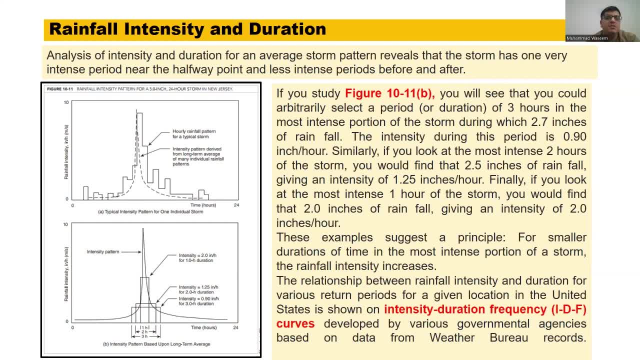 and if i move to two hours intense storm, then intensity is increasing like from 0.9 to 1.25 inches, and if i go towards one inch one hour uh intense storm, then intensity is like two inches per hour. so as you move towards uh intense period, like a short period, then its intensity will be. 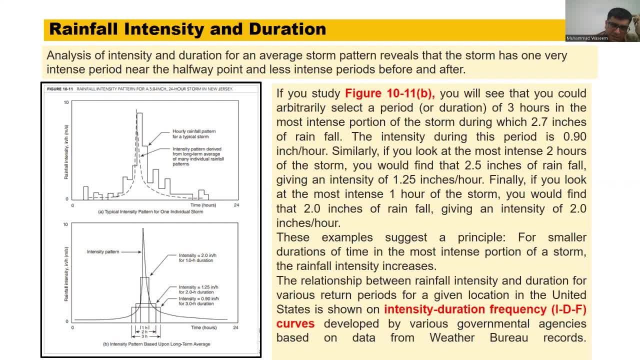 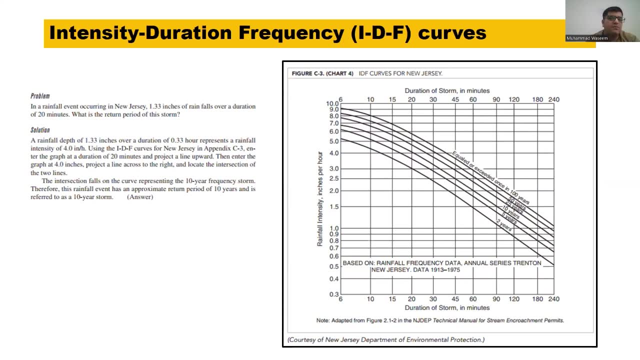 increased. so we we have, like uh, intensity, duration, frequency curves, which which shows the uh relationship between rate, fall intensity and duration. so here there is the rainfall intensity and duration of strong. so from here you can find the, the, basically the, the return period of storm. so let's say this is a rainfall of 1.33 inches. 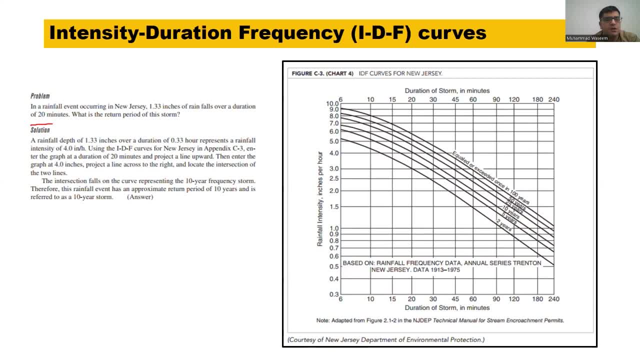 in 20 minutes, so in one hour it will be four inches per hour and it is for new jersey, so i have find the the idf curves for new jersey. so let's say four inches per hour. this is basically the four inches per hour and the duration of storm is basically 20 minutes. 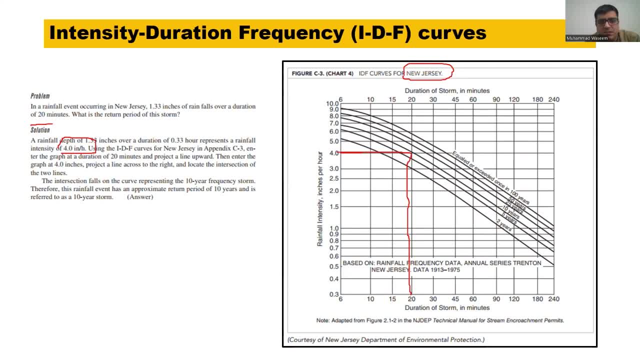 so this is the- or you can write this as 10 year return period- storm. so what you can see here is the return period for storm is somewhere straight line. this and this is your 10 year return period- strong. so this is how you find the return period for a particular rainfall intensity and duration: storm. 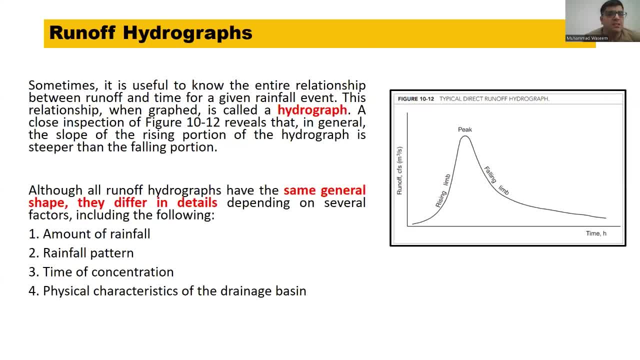 uh, through the intensity duration curves. now the next topic is basically the runoff hydrograph. so runoff hydrograph is basically the, the. it is useful to know the entire relationship between runoff and time for a given rate volume, and then when we plot this, this is called a hydrograph. so if you closely inspect this diagram, 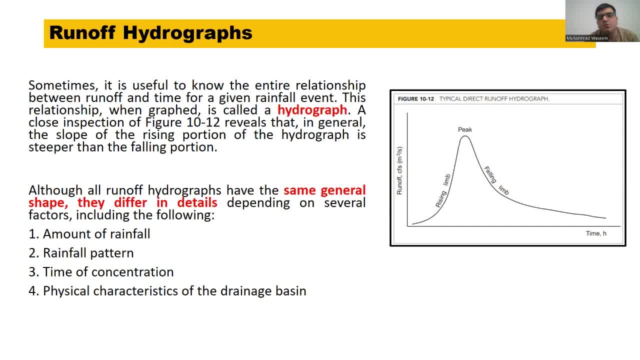 of 10-12, you will find that the slope of the rising portion of the hydrograph is steeper than the falling portion. this is basically the characteristics of all the hydrographs. why this happens? because, uh, the overland flow is a quick flow. it takes like uh uh small time for the 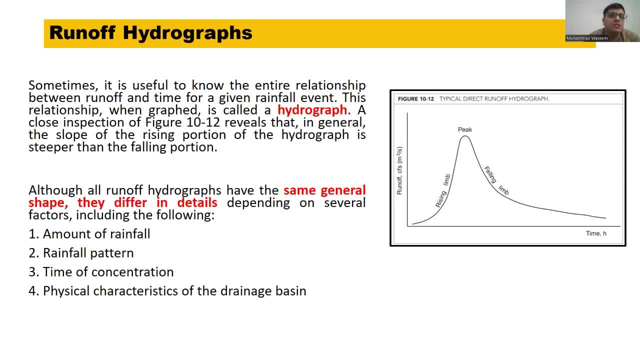 overland flow to reach from the remotest point to the, to the point of analysis, and then you will see the peak. but then there is a base. flow is also moving towards the, towards the point of uh, towards the point of analysis, but it takes larger time in comparison to the surface flow, so that 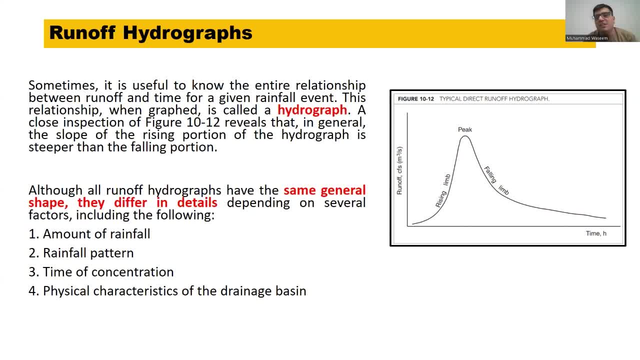 that comes slowly, so but when it reaches the peak is already gone. so that's why, when the base flow combines with the surface runoff or overland flow, then uh, the peak, at that time the peak is already gone. so that's why the but the, the gum water flows more gradually and slowly. 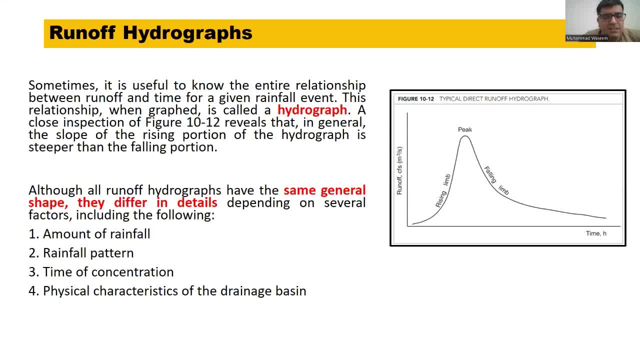 so that's why the falling leap is not that steep that it does not decline the flow steep after the rainfall event or after the peak flow. so the? although the all hydrographs have same channel shape, they differ in detail based on the amount of rainfall, rainfall pattern, time of 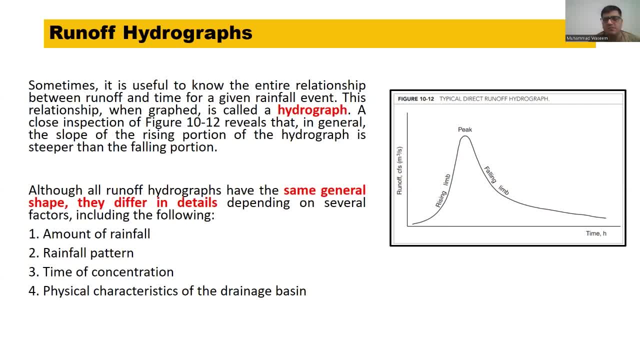 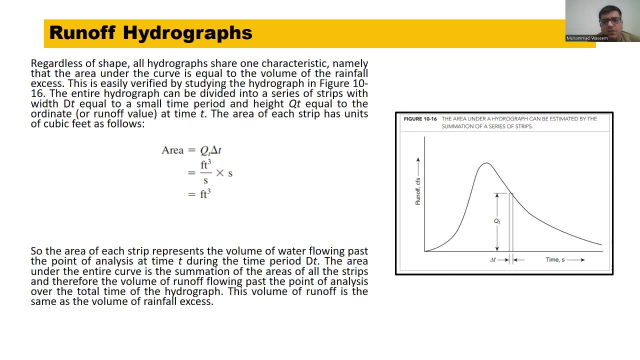 concentration and the physical characteristics of the drainage basin. so, uh, one thing: you need to know that the area under the curve is basically the volume. so how? so? let's say, if, if i divide this graph into smaller strips, so if, if i want to divide this graph into smaller strips, so if, if i want to, 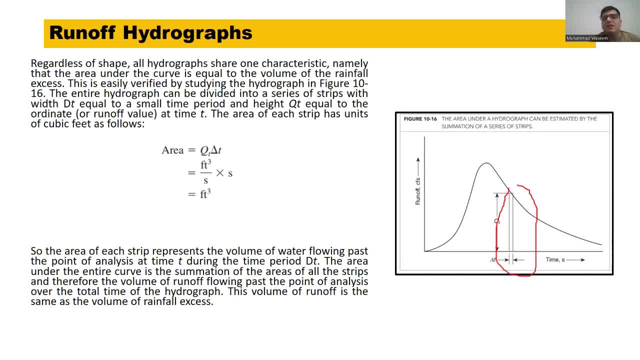 take the area of this street. this is basically area, is depth into width, so delta t multiplied by qt. so this is the basically the area. so qt is is that it has the unit of cubic feet per second and time is also in seconds. so the area is basically the volume, so area under each strip. 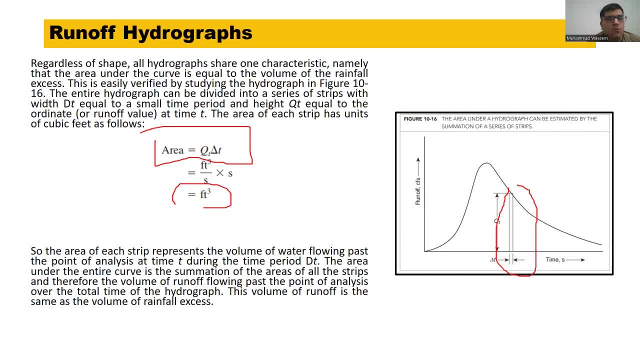 has, represents the volume of the water. so the area of each strip represents the volume of water flowing past the point of analysis at time t. so you want to take the area of this stream during the time period dt. The area under the entire curve is the summation of the. 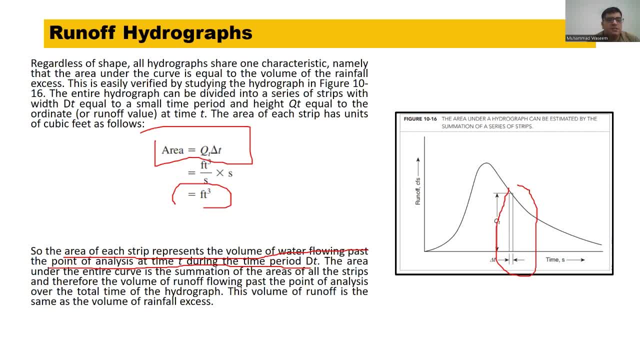 area of all these streams. So the volume of runoff is the same as the volume of excess rainfall. So this is basically how you find the, the rainfall, and then this, this curve which is basically between the runoff. this is this: runoff is direct runoff, that that is, the water in the streams, like if there is a 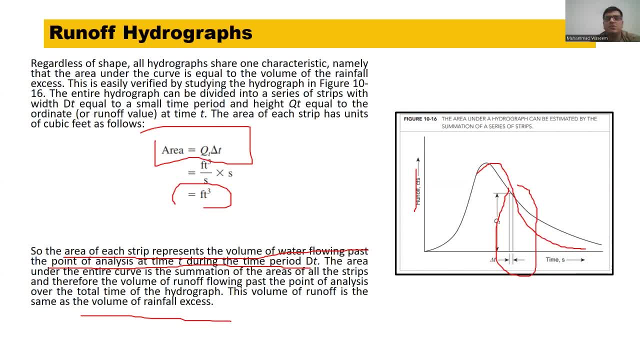 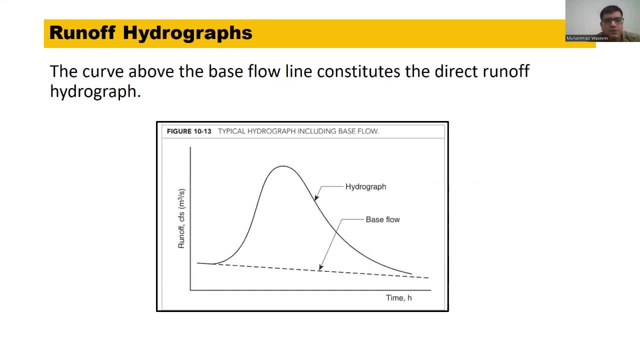 rain. if there is a gauge to flow the stream flow, this, this, this is that stream flow is basically direct runoff. So this runoff hydrograph also includes the base flow, because I have said said that the surface runoff will surface runoff, or the overland flow will also move towards the river and then the base flow. 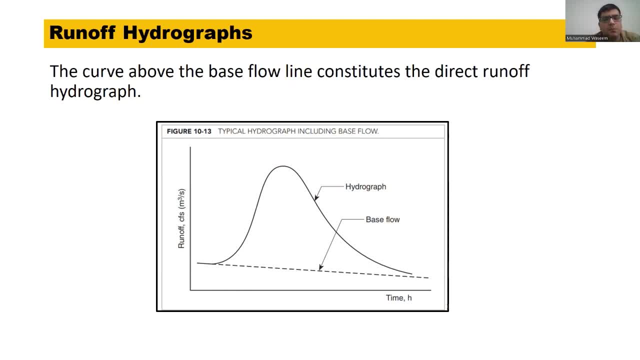 will also move towards the river. So this hydrograph is basically the combination of direct runoff and the base flow, Surface runoff or the base flow. so when I have to separate the direct runoff from the base flow, then then there are different methods. there is a software called pfi plus 3.0 you can use. 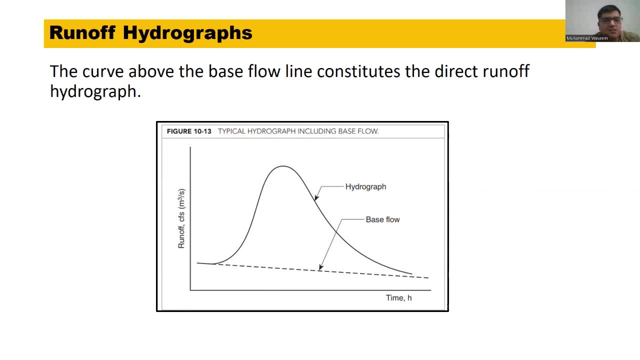 that to. it has different methods how you can separate hydrographs for direct runoff and base flow, but the simple method is you just combine these rising limb starting point to the falling limb and then the area under this portion is basically the base flow and that is area. 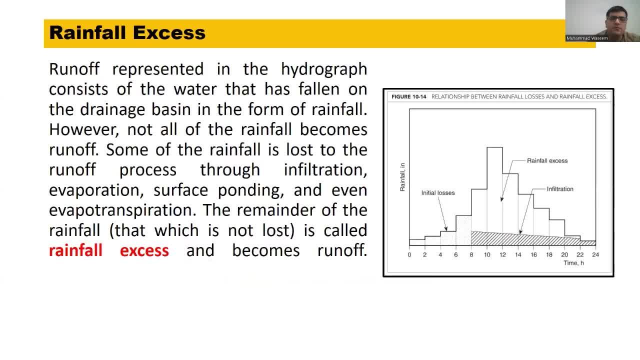 above that is called the direct runoff. So then I have explained that the direct runoff is basically the combination of overland flow and the sub and the subsurface flow. So, and these, both the flows- originates due to rainfall, but when the rainfall happens, not all the rainfall becomes runoff. some of the rainfall is lost due to during. 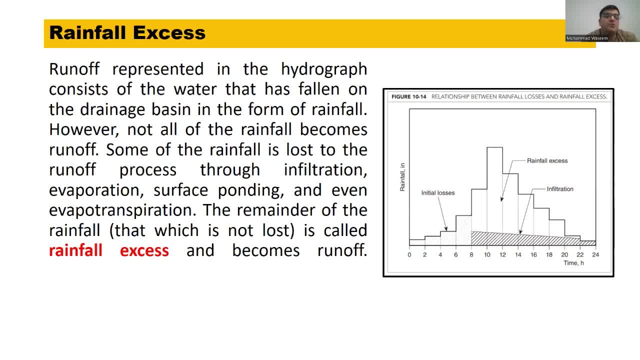 runoff processes to infiltration and evaporation. it could be either ponding and even evapotranspiration, so the rainfall that becomes the part of runoff is called the rainfall excess. So here in this diagram you can see this is the 24 hours time in the initial eight hours, whatever the rainfall was. 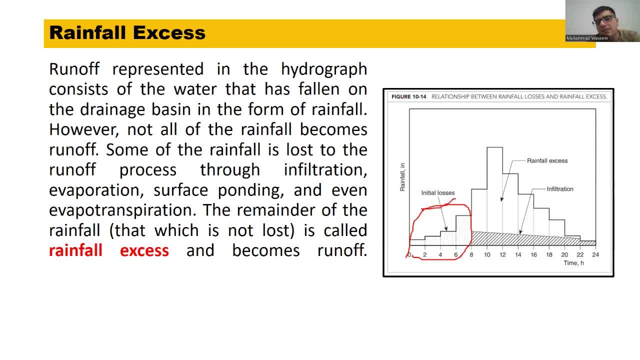 it was the losses, and then, when these losses were fulfilled, then the runoff started and then this runoff was also divided into base flow and also the rain surface flow. So this is the representation that this is the infiltration. so it will move towards the river as a base flow and then this will move towards the direct flow, and all of this. 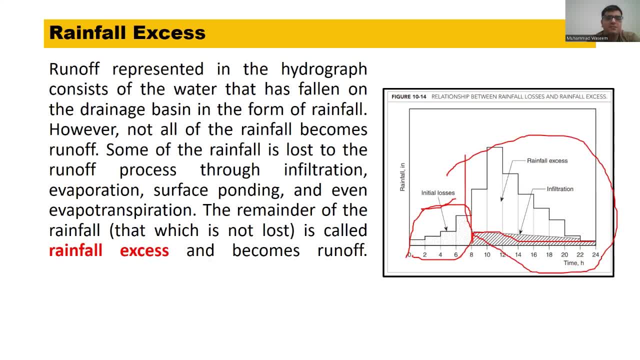 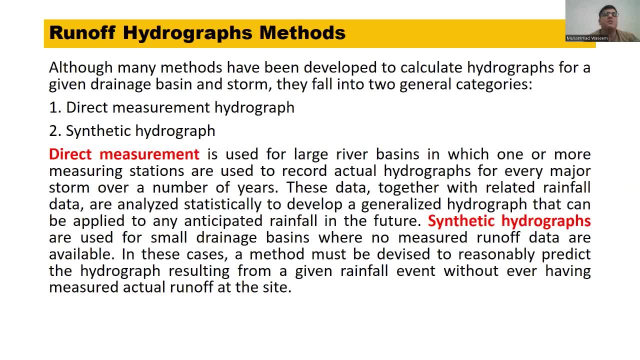 thing is based on the excess rainfall. The rainfall that is that becomes the part of runoff is called the rainfall excess. There are different runoff hydrograph methods- hydrograph methods like direct measurement hydrograph, synthetic hydrograph- so we will study them later in this course. the direct measurement run of hydrograph. i will explain you just remember. 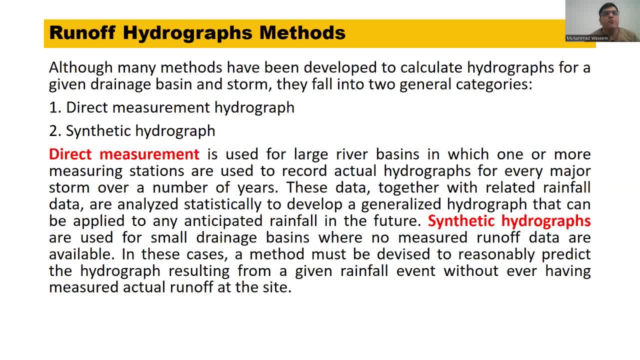 that is used for large river basins, when, where one or more main stations are used to record the actual hydrographs, right and synthetic hydrographs are used for small drainage basin where there is a no measured runoff data is available. in these cases, the method must be devised to reasonably. 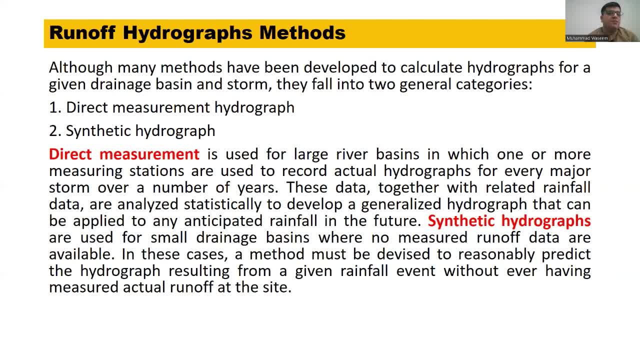 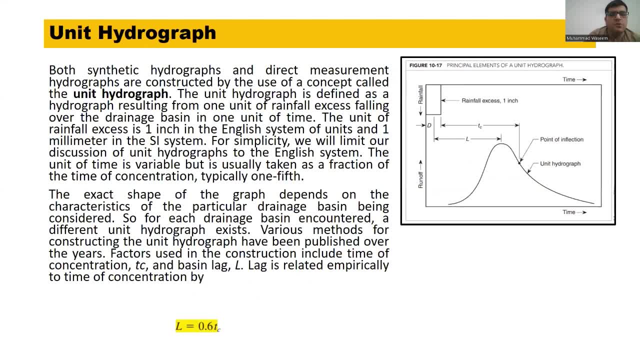 predict the hydrograph resulting from a given rainfall even without having measured actual runoff at the site. so unit hydrograph? what is unit hydrograph? so if? uh, let's say now we know what hydrograph is. hydrograph is basically a relationship when you plot the runoff versus time. that is called 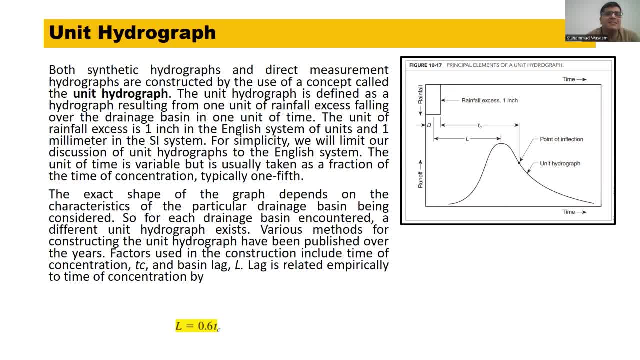 the hydrograph. so what exactly is a unit hydrograph? right? both synthetic hydrographs and direct measurement hydrographs are constructed by using the principle of unit hydrograph. so unit hydrograph you have to define. it is resulting from a one unit of rainfall excess falling over the drainage basin in. 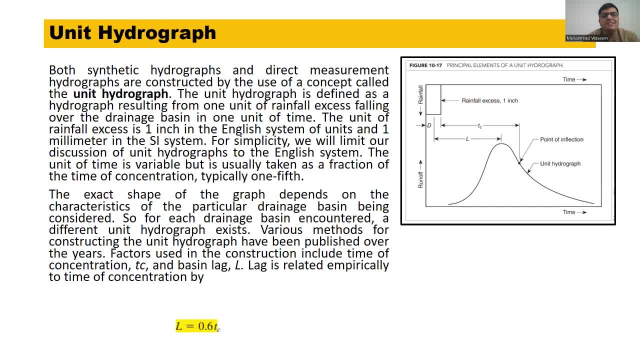 one unit of time. the one unit of rainfall excess is one inch in english system of units and one millimeter in si system of units. so, uh, basically the unit of time is variable, but it's really taken as a fraction of the time of concentration, typically, uh, typically one-fifth. let me just open one thing. 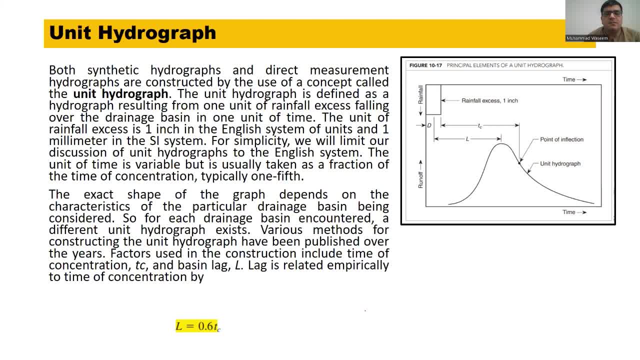 right. so let's say we study this uh diagram here. here there is a rainfall which is plotted on secondary axis in and uh, and this is basically the excess rainfall of one inch. right, then we have the runoff. so for this excess rainfall of one inch there will be, let's say there is a rainfall, and then the result of the rainfall will be a runoff. 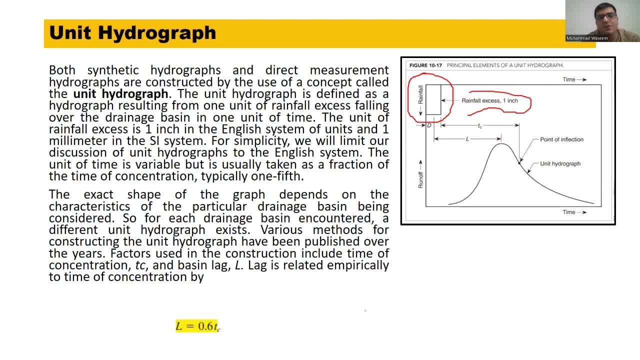 hydrograph, not a hundred run of hydrograph rainfall and runoff. so when we plot that runoff at any point of analysis, then this was the curve of that runoff. so from the center of excess rainfall to the peak is called the lag time, which is basically normally it is 0.6 into the time of. 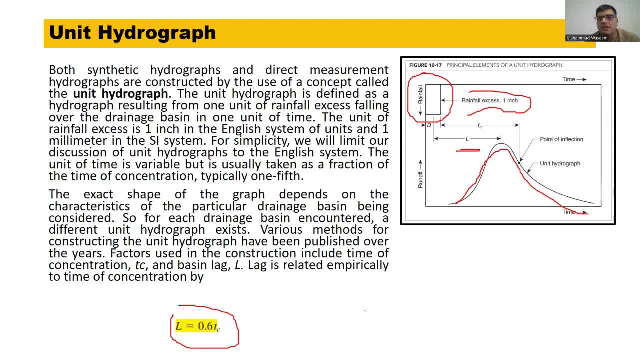 concentration, and time of concentration is basically when the rainfall ends, when the, when the uh rainfall ends, the, not the rainfall, excess rainfall, and it's from that, in that moment, the water from the remotest point to reach the point of analysis called the time of concentration, and it is normally after. 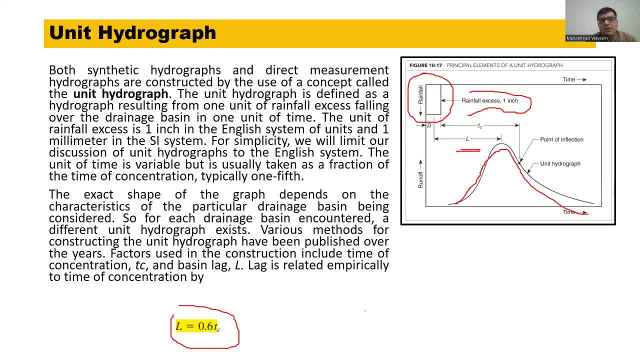 it reaches after the peak is gone. so that's why the time of concentration starts from this point at the end of the excess rainfall, and it leads towards the uh somewhere after the peak, at the point of, and that point is called basically the point of infection. so this is the unit hydrograph. 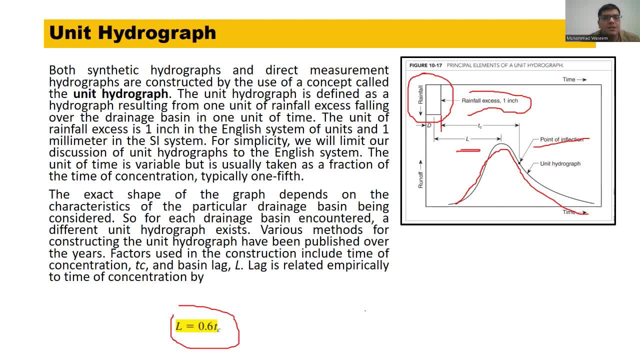 so what basically the purpose of unit hydrograph? let's say you have draw the for a particular attachment, for each different for each catchment there will be a different unit hydrograph for a unit rainfall right, let's say, in my area- i am currently in suvabi, in in the industry section. 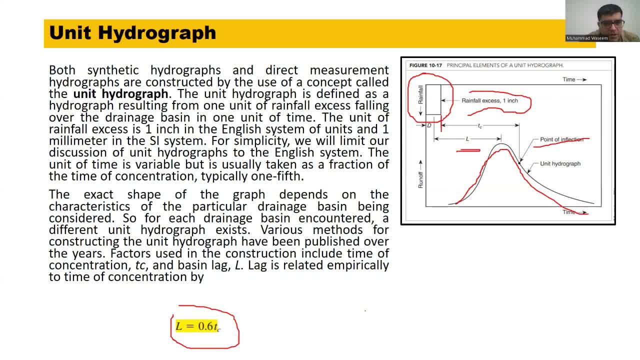 of uh catchment. let's say, if i know the rainfall for a particular rainfall, let's say unit rainfall- i know the unit hydrograph, the, the runoff basically, which will reach to the river. so let's say, if there will be 1.5 times the, 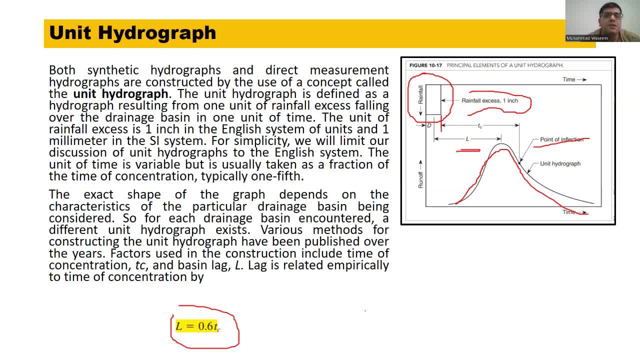 rainfall of that, then i will simply multiply this, so, uh, hydrograph with a factor of 0.5, 1.5, and then the new hydrograph i will obtain. so i don't have to go to the gauge and measure the peak. so this is the purpose. so you can, or you can, super position different hydrographs to find that. 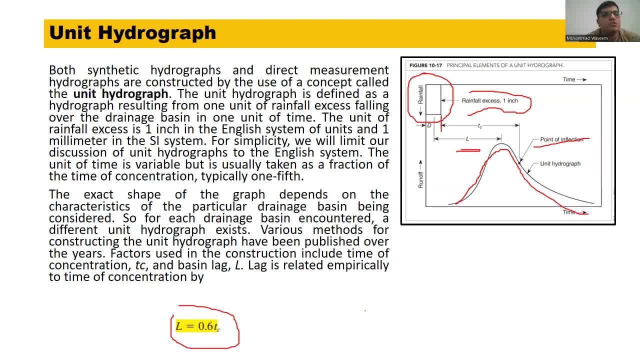 find your. uh, you can superposition different unit hydrographs to find your runoff hydrograph. so there are some assumptions. don't be confused. i will explain you what is the principles and how you multiply this and how you merge this. so i will explain you this slide just. 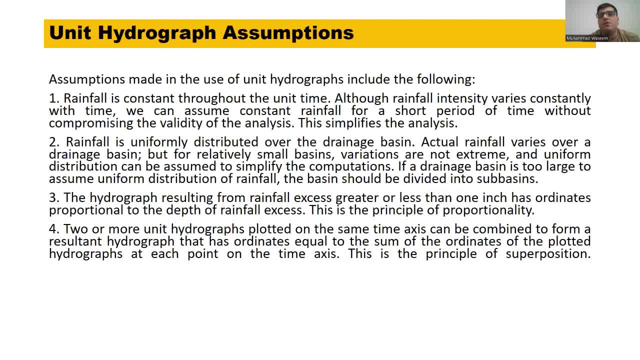 a moment. so this is. there are some assumptions. first, for the unit hydrograph. the first thing is that the rainfall is constant throughout the unit time. this is the main assumption, that throughout the unit time the rainfall is constant. then the the next assumption is the rainfall is uniformly. 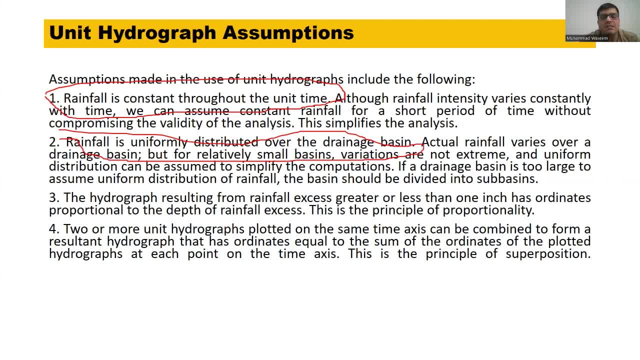 distributed over the drainage basin. so, uh, it's not that in the entire basin, the somewhere you know of this particular unit, uh, rainfall distribution is different in the other part is different. so it is distributed uniformly over the whole drainage basin, uh. and the third one is the 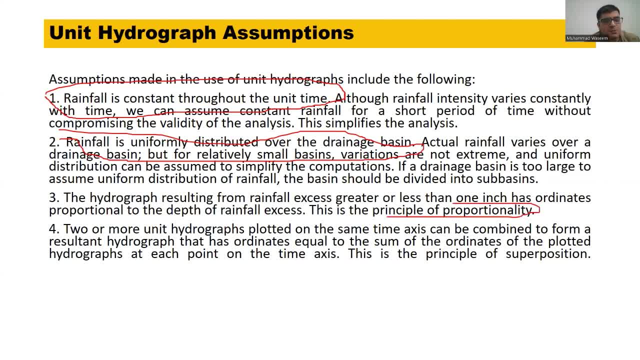 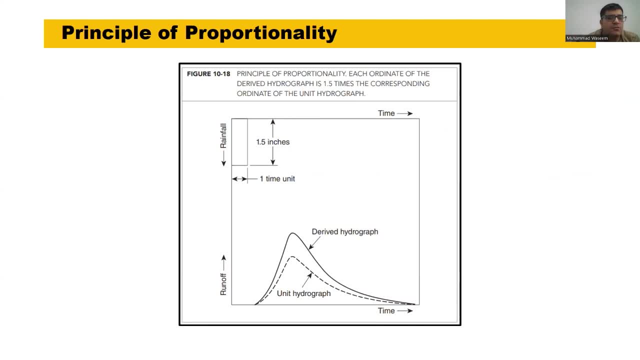 principle of proportionality and the fourth one is basically the assumption is the principle of superposition. what are these principle of proportionality and what is the principle of superposition? i will explain you in the next slides. let's say, in the previously i have explained you the, the, that for a one inch. 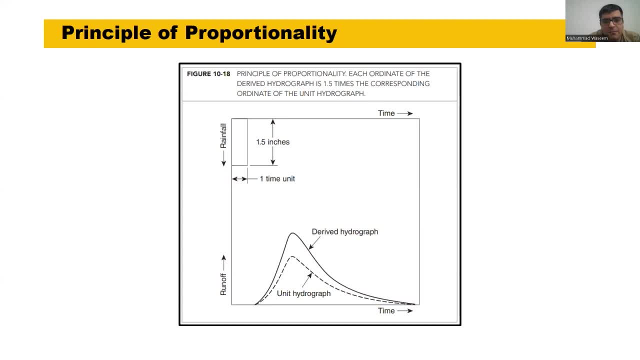 rainfall, which is basically our unit rainfall in a unit time. we have derived our hydrograph unit hydrograph, now, in this case the, the rainfall is not now the one one inch, it is one point five inch. so what we did? we multiply our unit hydrograph with a factor of 1.5, and then you got. 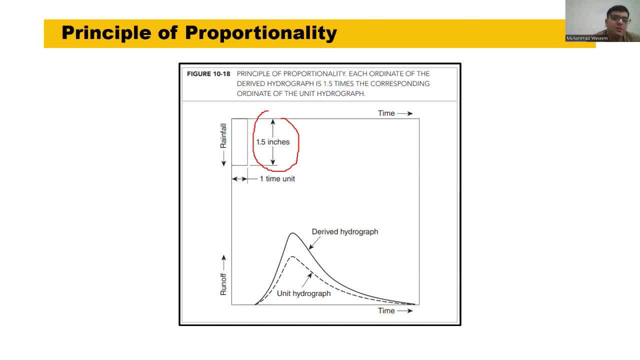 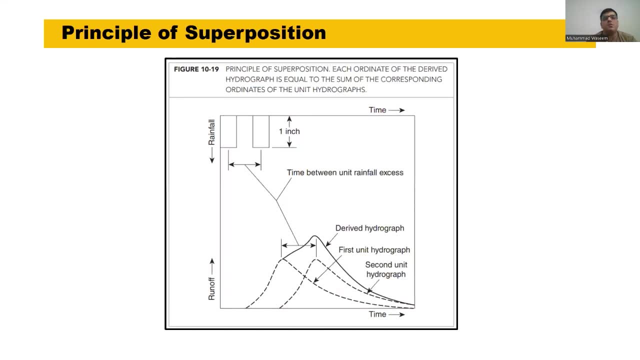 the dive hydrograph, you will see that the peaks will be aligned. so this is basically the principle of proportionality. and now, if you talk about the principle of superposition, uh, here, here is the scenario: that there is a one inch rainfall, then there is in the next hour, there is no rainfall. 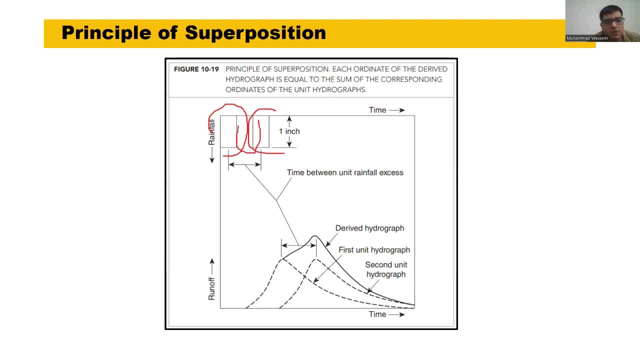 and then again there is a one inch rainfall. so for initial rainfall you have your hydrograph and then the other rainfall of one is you again have a same hydrograph, but the difference is basically the, the unit time between these two excess rainfall. so what we need to do you at this point where this hydrograph starts, so you just have to add. 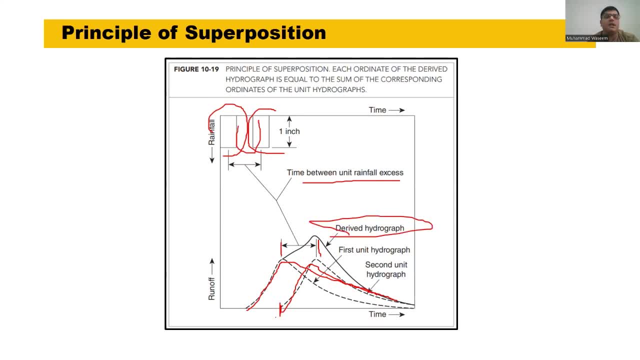 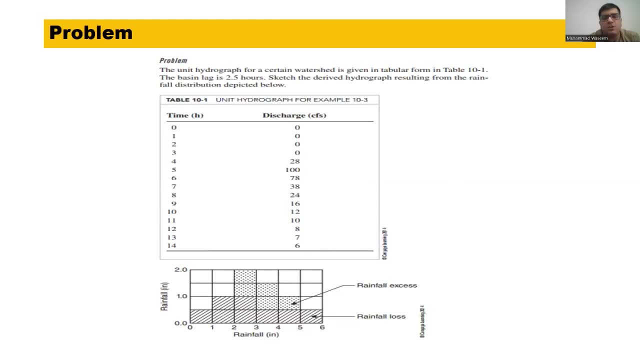 these, both hydrographs and you, you will find the new drive hydrograph. so this is how the principle of superposition works. now we have a problem. a unit hydrograph for a certain water shed is given in a tabular form in table 10-1. the basin is 2.5 hours, lag time is 2.5 hours. sketch the: 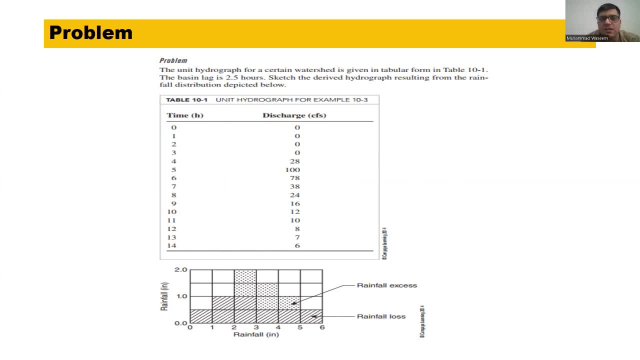 so what was the basin lag? so lag was basically the center of the excess rainfall to the peak. so sketch the drive hydrograph resulting from the rainfall distribution depicted. so this is the given data, that the discharge you know against the time and and you know the rainfall. so here, rainfall pattern. 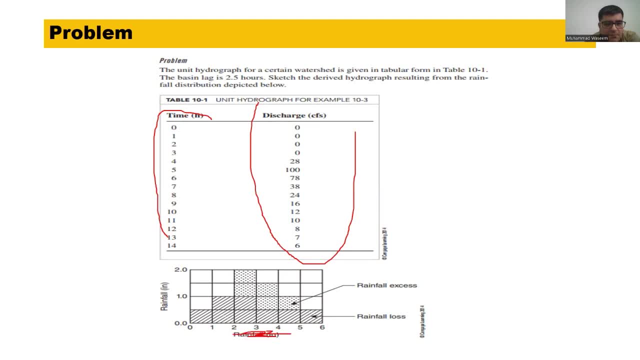 on it. there is a type of mistake. this is not rainfall. this is basically the time. so this is basically the time. so first hour there was rainfall, but it was a rainfall. it was a rain loss. in the second hour the rainfall was one inch, but the complete one inch rainfall was the loss. 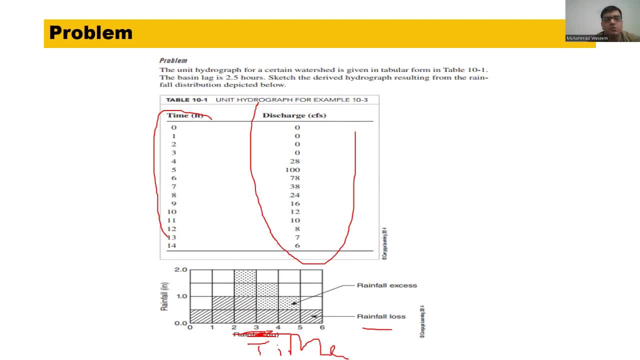 in the two to three. in the third hour the rainfall was two inch, but one inch was the rainfall losses and the other one inch was the rainfallемон impactoaku. in the three to four hour period, the total rainfall was 1.5 inch and one inch was the 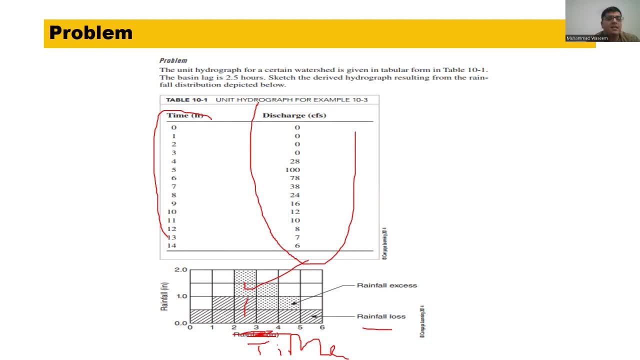 rainfall excess and the 0.5 inch was the rainfall loss. and then the next time period there was one inch rainfall, half was lost. and how was how was excess rainfall and the final interval there was rainfall of 0.5 inch and it was again the rainfall loss. so if you study this, you will see then there. 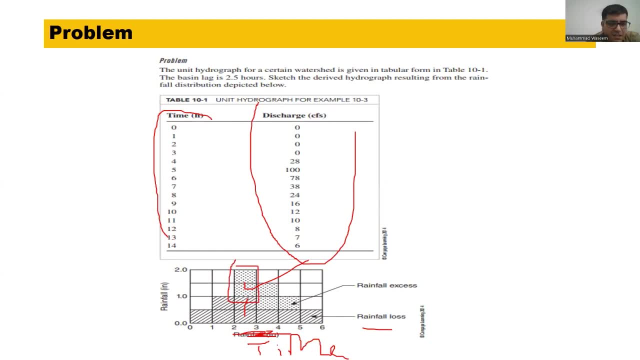 is a one, one inch rainfall excess, then again there is a one inch rainfall excess, and then there is a 0.5 inch rainfall excess and this is basically the discharge which is given to you, which was observed at the point of this is basically the unit hydrograph discharges, right, which you have. 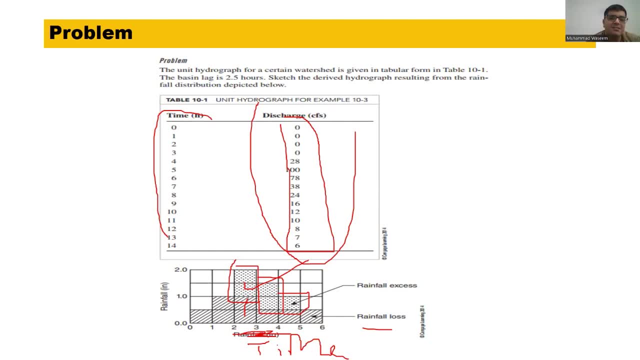 prepared and now you have from this unit hydrograph. against this rainfall distribution. you have to find the runoff hydrograph, not the unit hydrograph. unit hydrograph is for the unit rainfall right. this is for the unit rainfall, which is basically one inch. so here in this first portion, the rainfall is one inch. 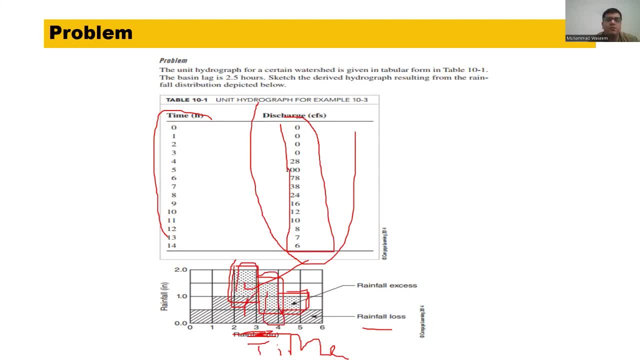 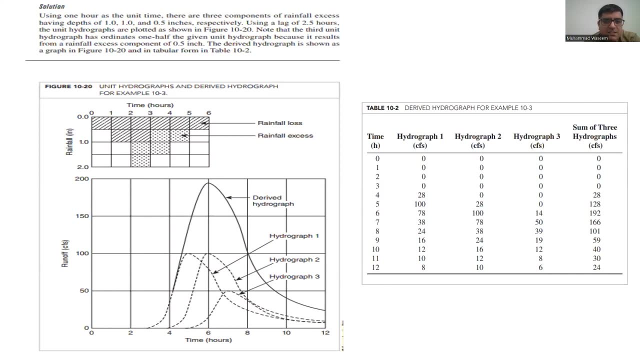 here it is again one inch and there is 0.5, so for one inch the rainfall will remain same. so let's say we move towards the solution. so runoff hydrograph, as it is equal to unit hydrograph, so it is same. then there is a difference of one hour, so these values will move to the 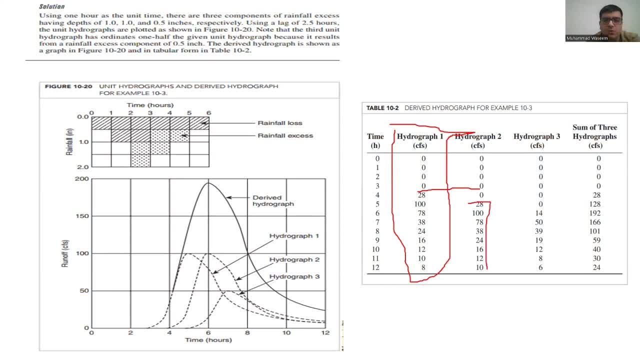 one hour later. so for these two, both runoff hydrograph, as these were same as unit hydrograph- and then the unit hydrograph number three, which was basically for this rain, which is 0.5, so we half the values, so for and it will move again one hour later. so 14, uh, 28, half 14. 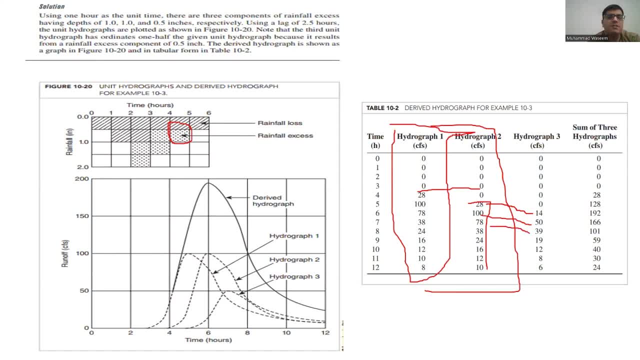 100, half 50, 78, half 39, and then you sum all these hydrographs. you will get the uh runoff hydrograph. so if you plot this time versus this sum of these three, then you will get this drive runoff hydrograph. so this is how you basically draw your hydrocaps. i hope you haven't. 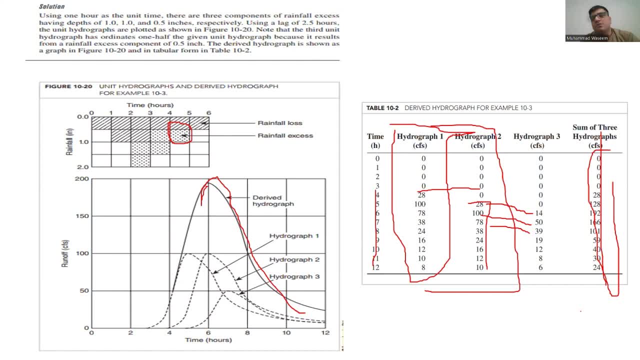 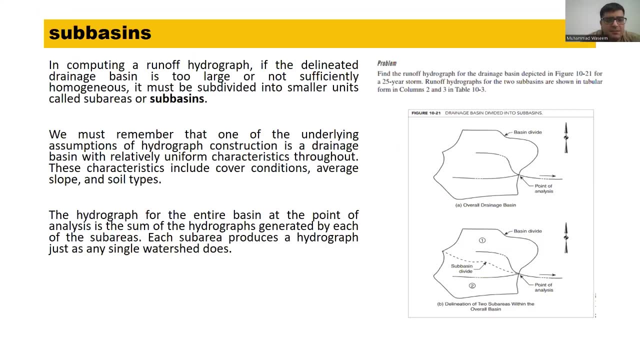 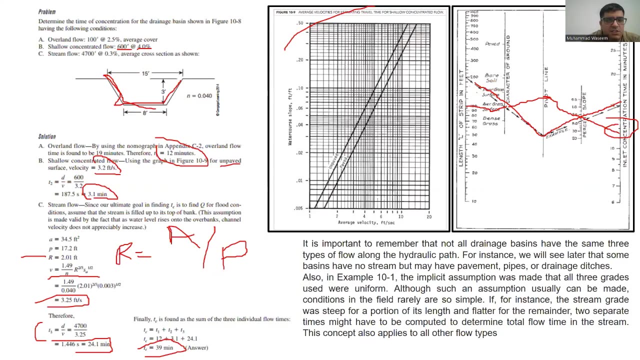 understood if you, if you uh have any question, you can write in the comments or you send an email. so now about the sub business. uh i, when we were studying this slide and the- i think the figure here, i have told you that. then the whole business: initially, 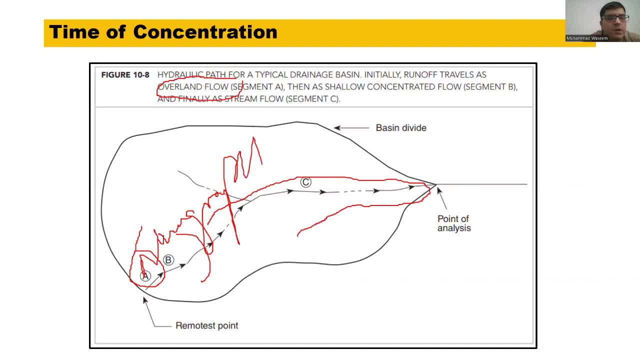 uh, there was a well and flow, then shallow concentrated flow and the finally there was stream flow. but i have told you that in reality it is difficult, that it's not nearly impossible that that for entire basin there will be initially a overland flow, because the characteristics of whole 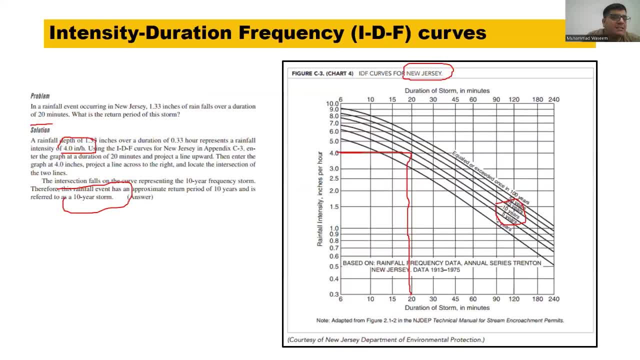 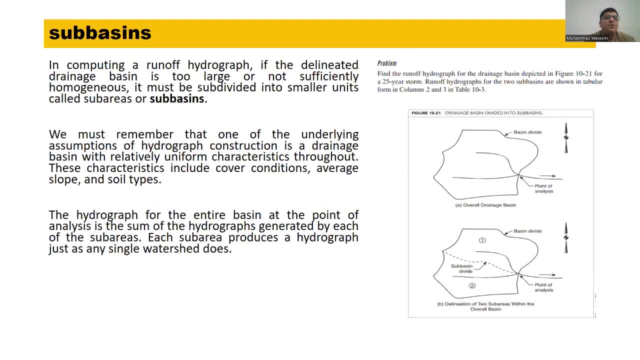 basin is not really the same. so what we do, that to analysis, to make things similar in in the entire uh, catchment we, what we do, we divide the basin into into smaller sub business where the characteristics are more or less same. so here in this let's say this was the business, complete this, and there are 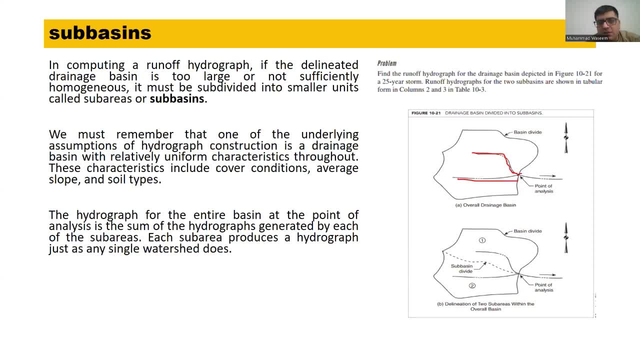 two rivers- one is this and one is this- where they merge is called the point of analysis or the point of confidence. so at this point we delineate the catchment and then we divide it into two subways, and one is number one and the other is number two. 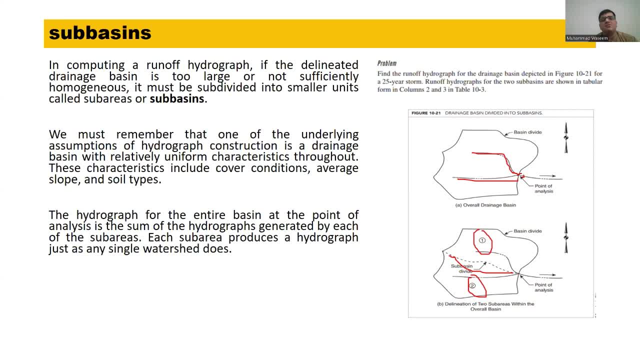 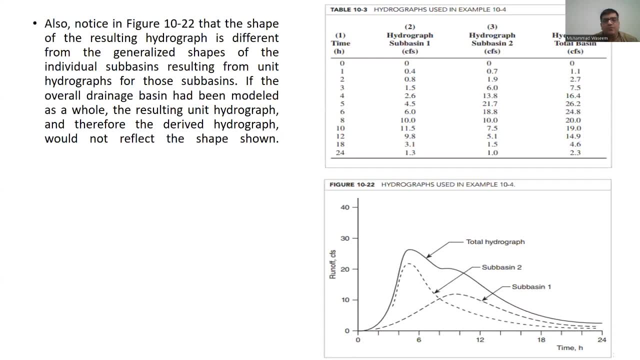 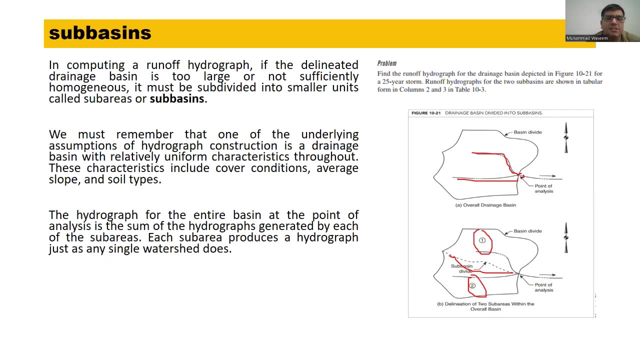 so now the characteristics of sub basin one is same and the characteristics of sub-dison two is the same. so next there is a uh. if you uh, there is a like problem. find the run up hydro graph for the drainage basin depicted in figure 10-21 for 25 years strong. the hydrographs for the two. 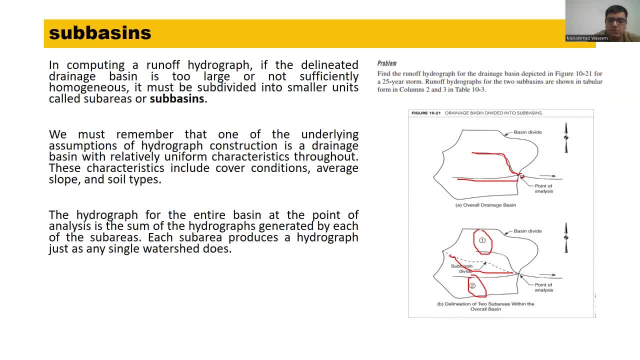 sub-disons are showing tabular form in column 2 and 3 in table 3.. so column 2 and 3 in table 3, table three. So these are the runoff hydrogas for. So what you need to do is you just have.